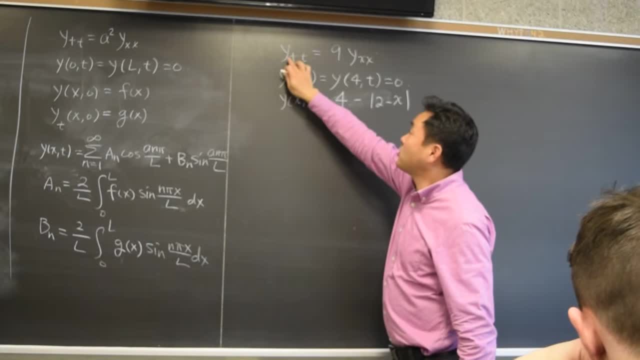 let me explain what's going on here. I explain that this type of. let me explain what's going on here. I explain that this type of equation is a wave equation. that if equation is a wave equation, that if equation is a wave equation, that if you take the second derivative of the, 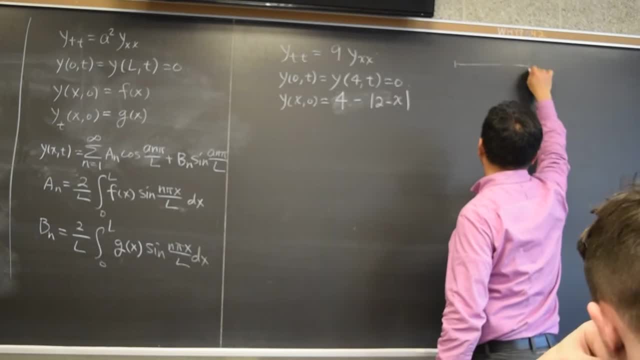 you take the second derivative of the. you take the second derivative of the position. think about the string that's position. think about the string that's position. think about the string that's tied at the end and you're trying to tied at the end and you're trying to. 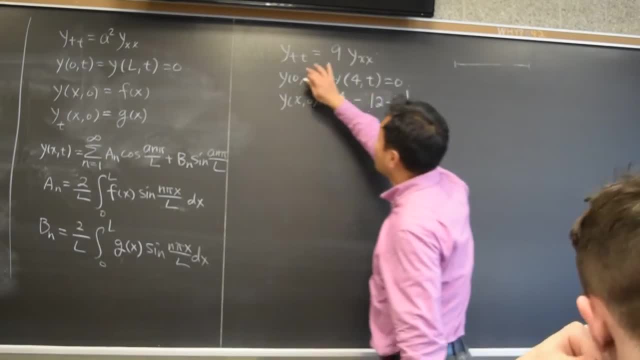 tied at the end and you're trying to vibrate this, this string. if you take the vibrate this, this string, if you take the vibrate this, this string, if you take the second derivative of the y position, then second derivative of the y position, then second derivative of the y position, then that's the acceleration in the y. 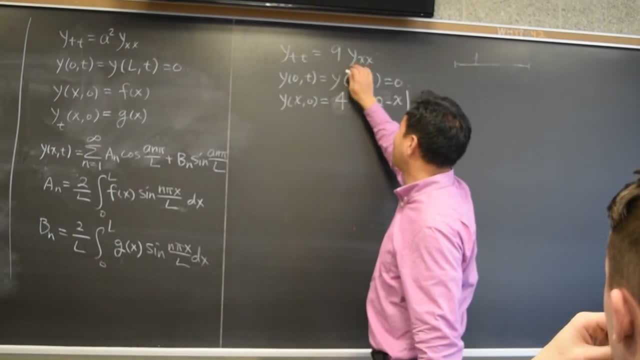 that's the acceleration in the y position, then that's the acceleration in the y, that's the acceleration in the y direction. right, and it's basically saying direction right, and it's basically saying direction right. and it's basically saying that the way, the concavity, how it's. 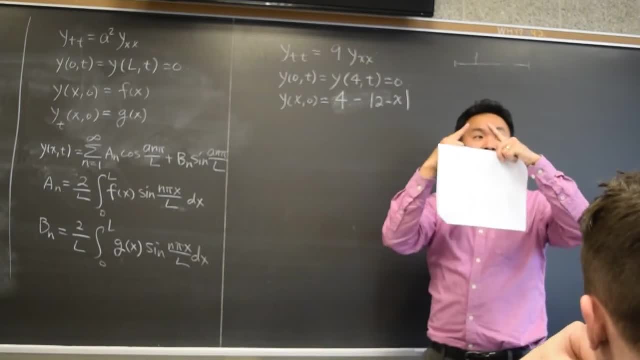 that the way, the concavity, how it's that the way the concavity, how it's bended, the more bended it is, the more bended, the more bended it is. the more bended, the more bended it is, the more force it will be acting on this string. 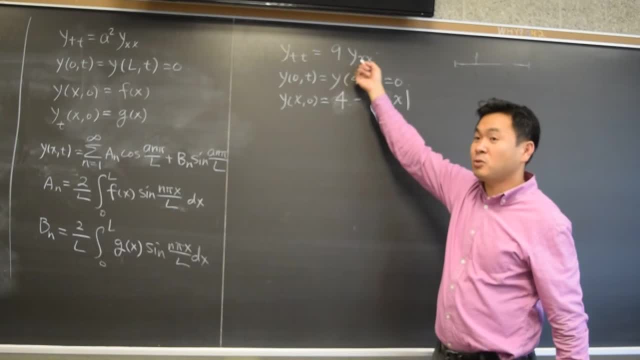 force. it will be acting on this string force. it will be acting on this string. right so yxx computes the bending, and right so yxx computes the bending. and right so yxx computes the bending. and times. some constant gives you the times. some constant gives you the. 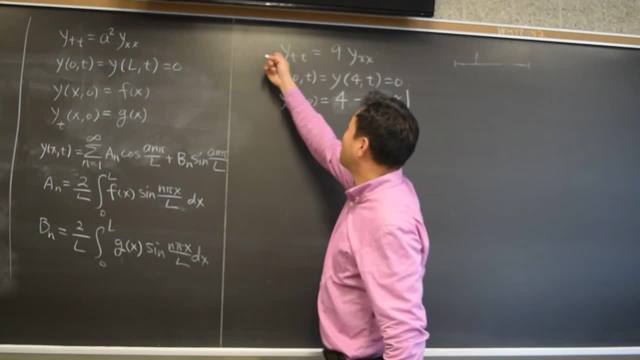 times some constant gives you the acceleration, but what's really here? acceleration. but what's really here? acceleration. but what's really here? hidden here is that it's really F equal. hidden here is that it's really F equal. hidden here is that it's really F equal to ma and M is here, but that M is. 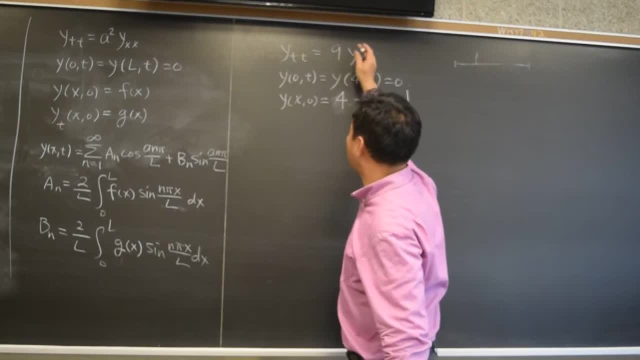 to ma and M is here, but that M is to ma and M is here, but that M is divided over here and it's along some divided over here and it's along some divided over here and it's along some. somehow it's a, it's a in this constant. 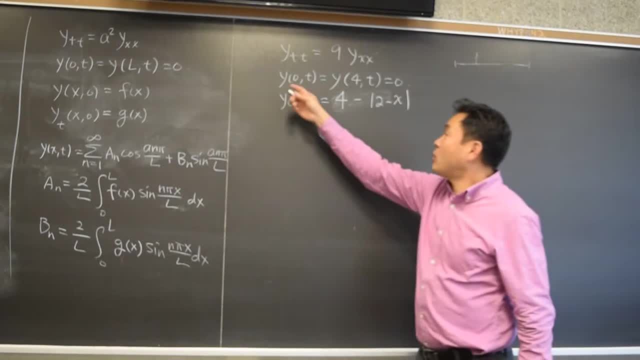 somehow it's a. it's a in this constant, somehow it's a. it's a in this constant: okay, all right. and here y of 0 T, okay, all right. and here y of 0 T, okay, all right. and here y of 0. T equals to y of 40. equal to 0 means that. 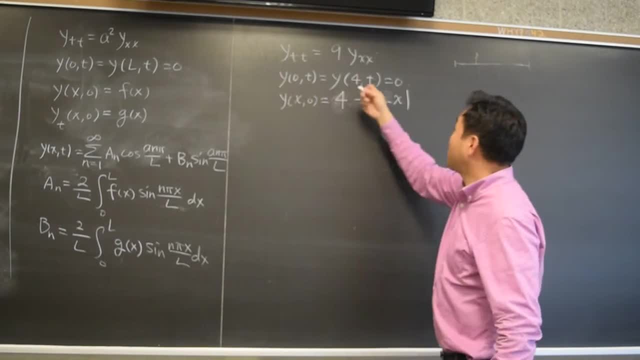 equals to y of 40 equal to 0. means that equals to y of 40 equal to 0. means that, for any time, the position at 0 and 4. for any time, the position at 0 and 4. for any time, the position at 0 and 4 are 0, which means at 0 and at 4. this 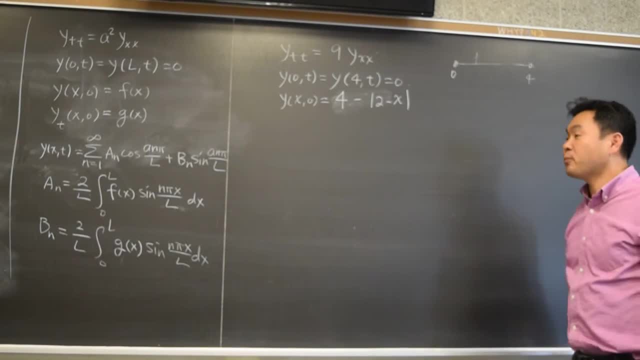 are 0, which means at 0 and at 4. this are 0, which means at 0 and at 4. this position doesn't change. meaning that the position doesn't change. meaning that the position doesn't change. meaning that the endpoints are always fixed. okay, and. 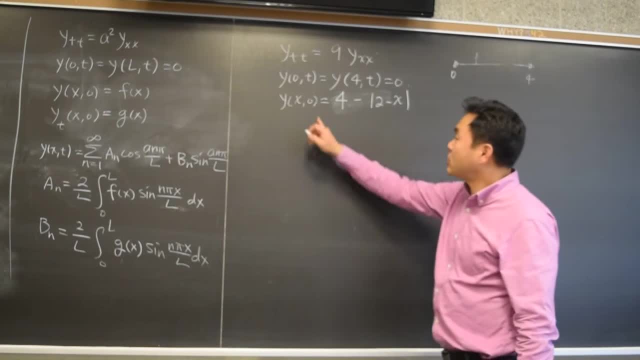 endpoints are always fixed. okay, and endpoints are always fixed okay. and then let's say y of X- 0 when initially. then let's say y of X- 0 when initially. then let's say y of X- 0 when initially, at time, t equal to 0, you have the 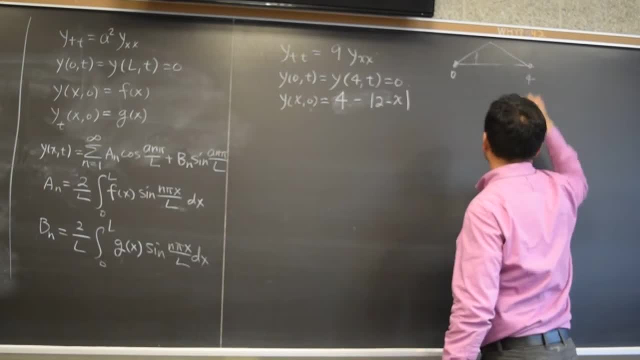 at time t equal to 0, you have the. at time t equal to 0, you have the following displacement: let's say you have. following displacement: let's say you have: following displacement: let's say you have this so that they'll be like: you take a. 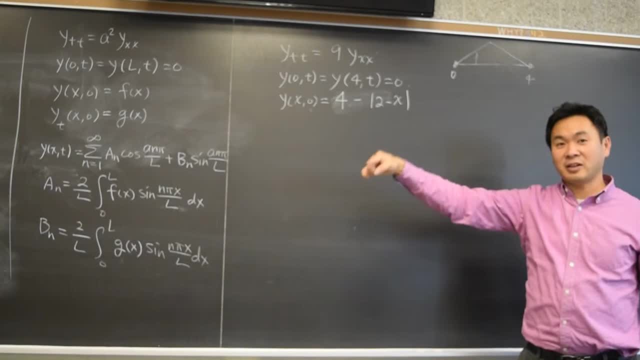 this so that they'll be like you take a this so that they'll be like: you take a string and you pull it at one point, so string and you pull it at one point, so string and you pull it at one point, so it's bended like that and you release it. 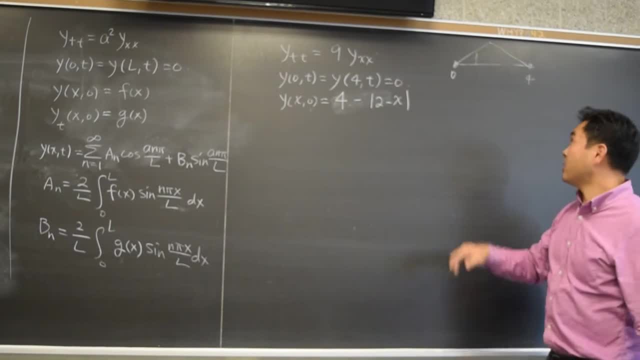 it's bended like that and you release it. it's bended like that and you release it, and then it's going to go back, and, and then it's going to go back, and, and then it's going to go back and forth. right, and that, that's what we want. 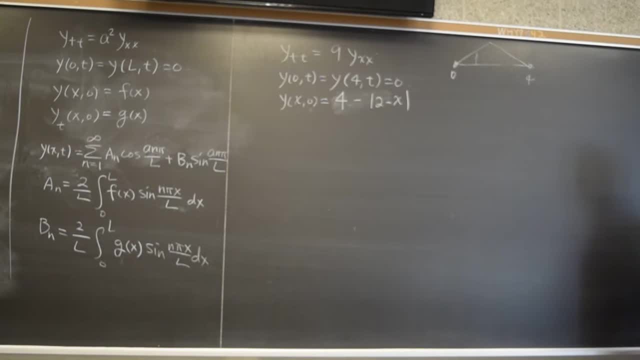 forth right, and that that's what we want forth, right, and that that's what we want to figure out now. it's actually to figure out now. it's actually to figure out now. it's actually interesting to choose to graph the. interesting to choose to graph the. 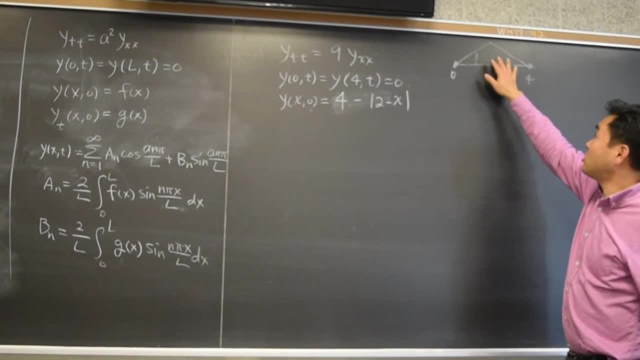 interesting to choose to graph the solution after you solve this, if you solution after you solve this, if you solution after you solve this, if you solve this and you see the graph of the solve this and you see the graph of the solve this and you see the graph of the solution. it, it always maintains this. 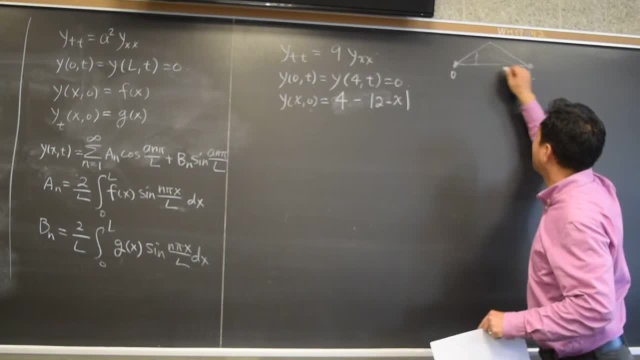 solution. it it always maintains this solution. it it always maintains this, this type of solution. it will do like this type of solution. it will do like this type of solution. it will do like then it would just go back and forth. then it would just go back and forth. 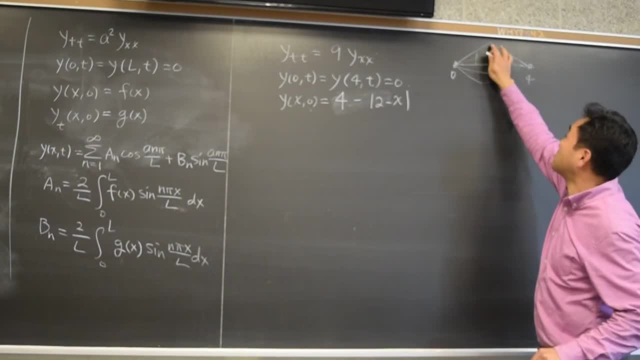 then it would just go back and forth, maintaining this is cusp- here the point. maintaining this is cusp- here the point. maintaining this is cusp, here the point that it's not differentiable, and that's that it's not differentiable, and that's that it's not differentiable, and that's not really the same thing as the reality. 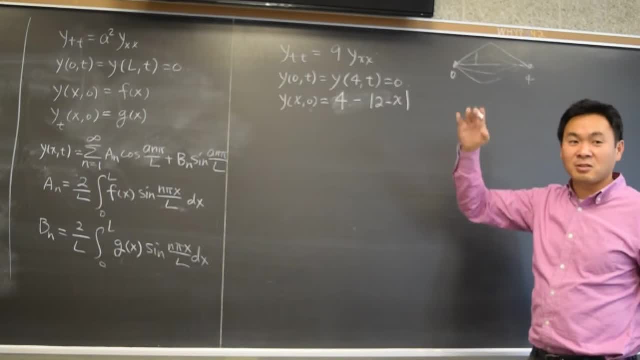 not really the same thing as the reality. not really the same thing as the reality. if you really took a string and you, if you really took a string and you, if you really took a string and you released it, then because some friction released it, then because some friction. 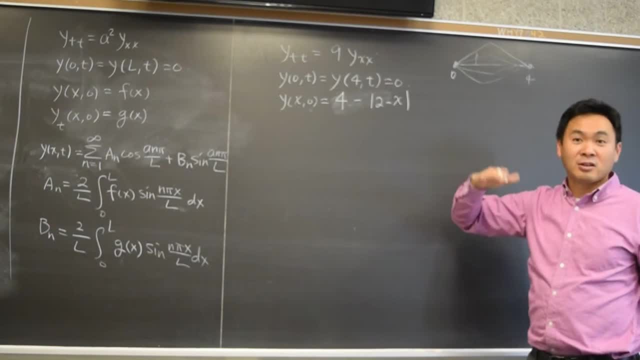 released it then because some friction, and actually you lose a lot of energy and actually you lose a lot of energy and actually you lose a lot of energy due to sound right and because of that, due to sound right, and because of that, due to sound right, and because of that it gradually becomes, reaches equilibrium. 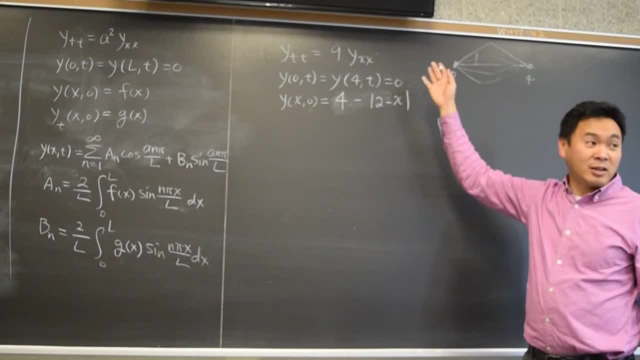 it gradually becomes, reaches equilibrium. it gradually becomes, reaches equilibrium. here it doesn't. it will always because. here it doesn't. it will always because here it doesn't. it will always because we don't assume any kind of friction. we don't assume any kind of friction. we don't assume any kind of friction when you've been released it the 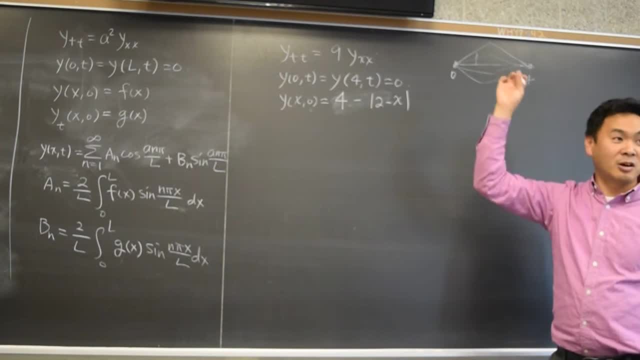 when you've been released it, the when you've been released it, the solution will will tell you that it goes. solution will will tell you that it goes. solution will will tell you that it goes back and forth without any loss in the back and forth, without any loss in the. 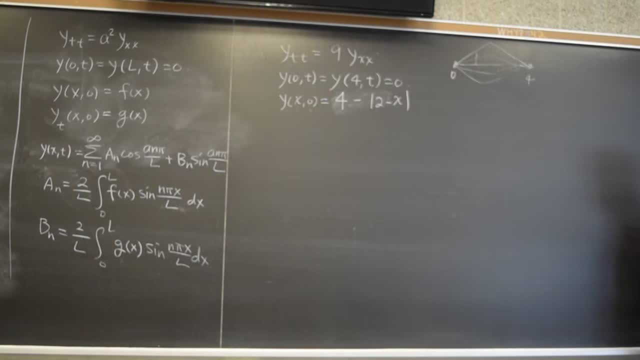 back and forth without any loss in the amplitude. okay. so that's kind of not amplitude okay. so that's kind of not amplitude okay. so that's kind of not what you would expect in the real life, what you would expect in the real life, what you would expect in the real life, but still it's, it's useful. so this is. 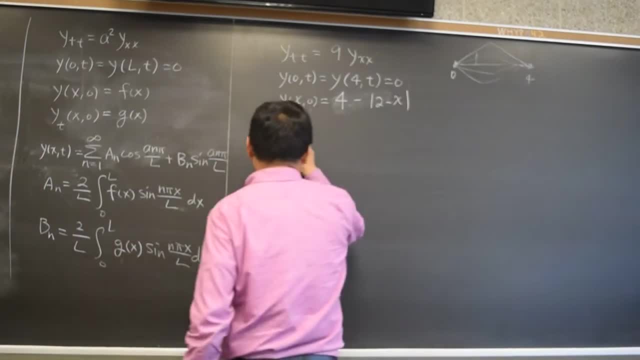 but still it's it's useful. so this is, but still it's it's useful. so this is called the wave equating and let's just called the wave equating and let's just called the wave equating and let's just say the initial speed, Y prime or Y T X. 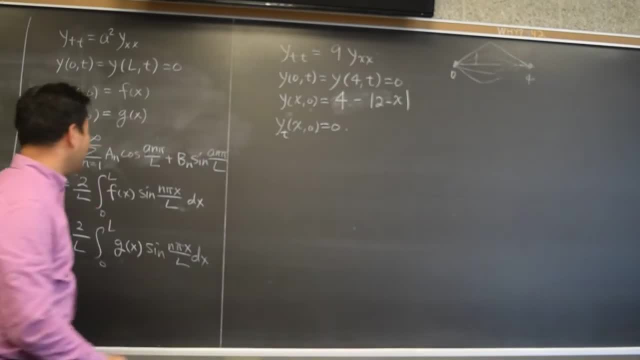 say the initial speed, Y prime or Y T X. say the initial speed, Y prime or Y T X. zero is zero. so then we don't have to: zero is zero, so then we don't have to. zero is zero, so then we don't have to calculate this. all right, so suppose. 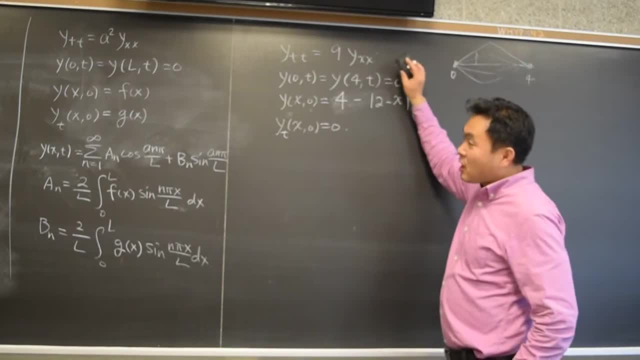 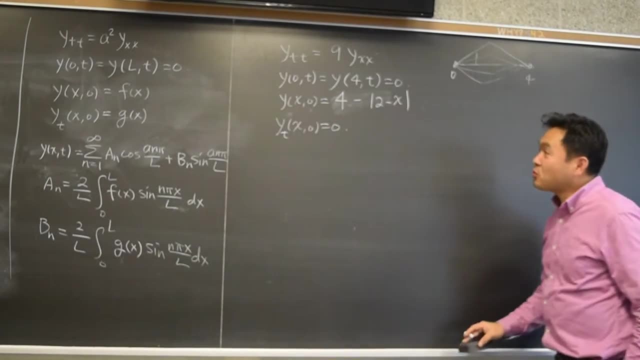 calculate this all right. so suppose, calculate this all right. so suppose you're given this problem and you're you're given this problem and you're you're given this problem and you're also given this formula, the formula also given this formula, the formula also. given this formula, the formula sheet. first you have to locate the 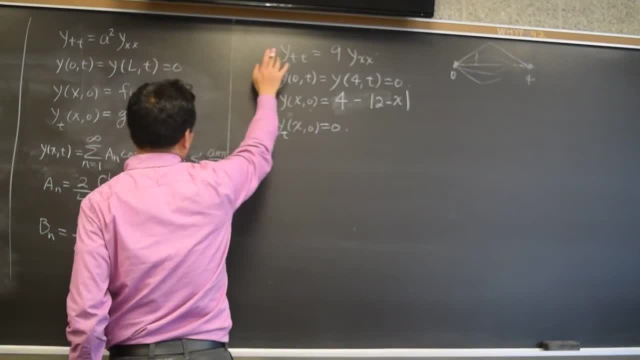 sheet. first you have to locate the sheet first. you have to locate the derivatives correct. locate the formulas- derivatives correct. locate the formulas- derivatives correct. locate the formulas and compare it and see if it matches you and compare it and see if it matches you and compare it and see if it matches. you have two derivatives in T, two there is: 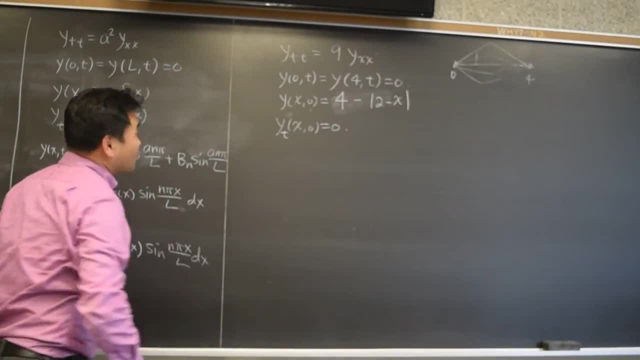 have two derivatives in T two. there is have two derivatives in T two. there is an X to do the next. so that means we are an X to do the next. so that means we are an X to do the next. so that means we are talking about the same wave equation. 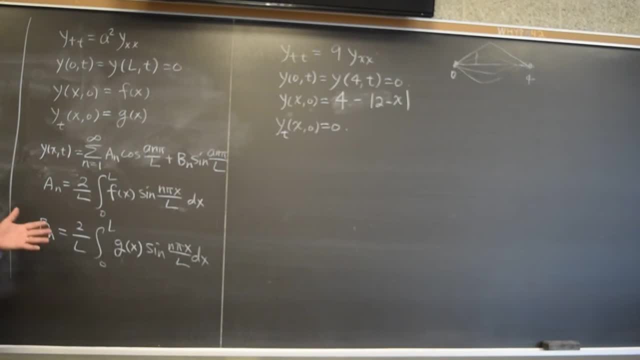 talking about the same wave equation. talking about the same wave equation. so let's say, you figured out that this is so. let's say, you figured out that this is so. let's say, you figured out that this is the, the equation that you want all, the, the equation that you want all. 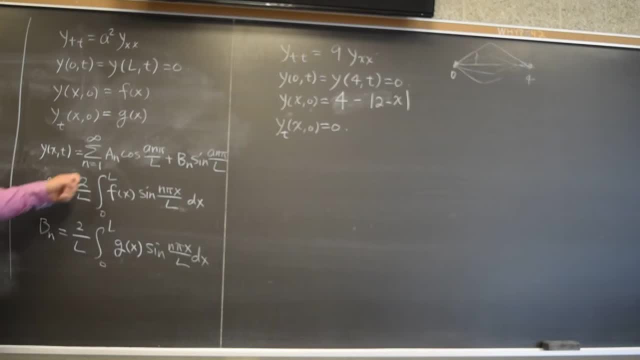 the, the equation that you want. all right, then we just compute this and plug. right then we just compute this and plug. right then we just compute this and plug it in here, and that's pretty much it. it in here, and that's pretty much it. it in here, and that's pretty much it. something's not right here in this. 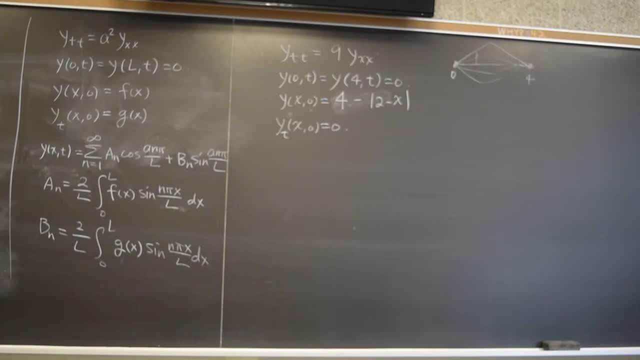 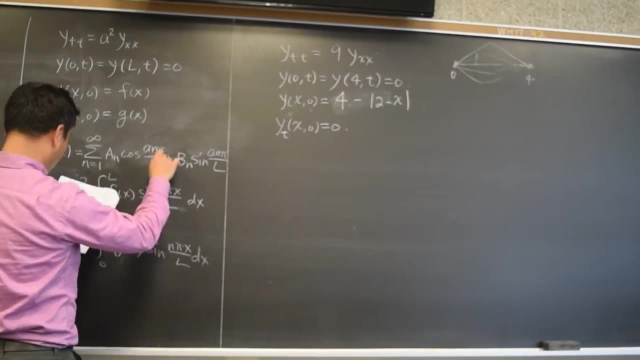 something's not right here in this. something's not right here in this. oh yeah, yeah, sorry, this is a. this is T in. oh yeah, yeah, sorry, this is a. this is T in. oh yeah, yeah, sorry, this is a. this is T in. there, there, there and. 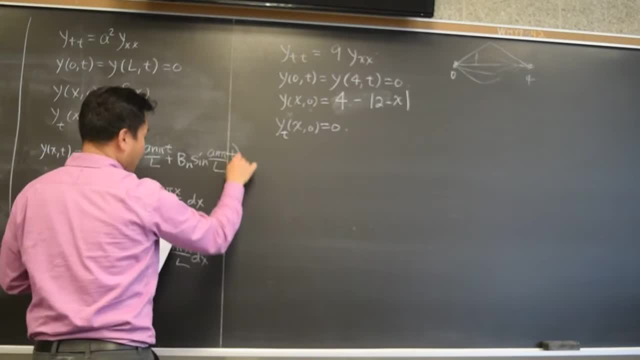 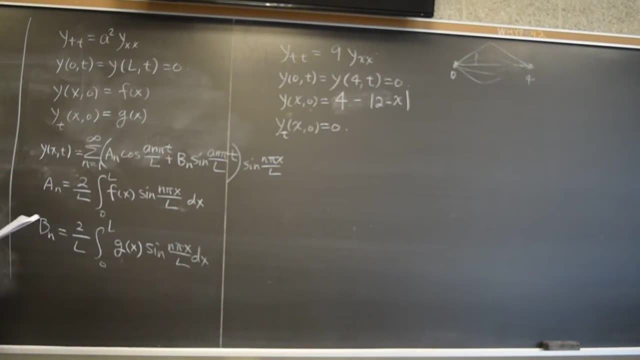 and and and and the entire thing should have sine. the entire thing should have sine. the entire thing should have sine. of n pi X over L. so I made a mistake in of n pi X over L. so I made a mistake in of n pi X over L. so I made a mistake in copy the formula. okay, so, given this, 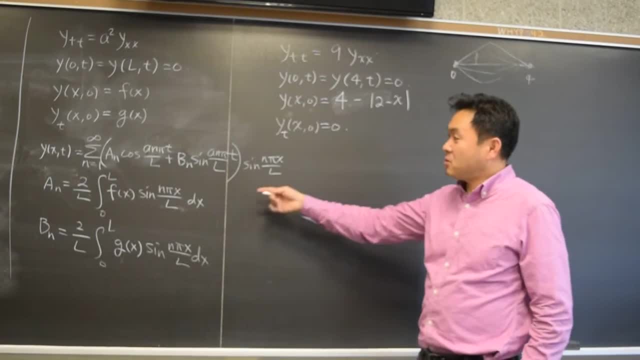 copy the formula. okay. so, given this, copy the formula. okay. so, given this formula, how do you solve this? well, you formula. how do you solve this? well, you formula. how do you solve this? well, you just use the formula. that's it, yes on. just use the formula. that's it, yes, on. 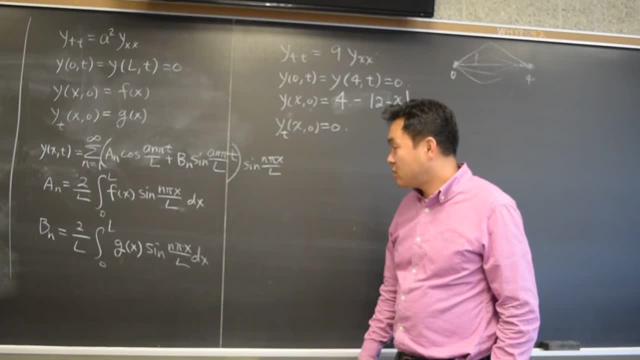 just use the formula. that's it. yes, on. here it says B n is equal to 2 over a. here it says B n is equal to 2 over a. here it says B n is equal to 2 over a n pi. oh, okay, so I right, right, right. 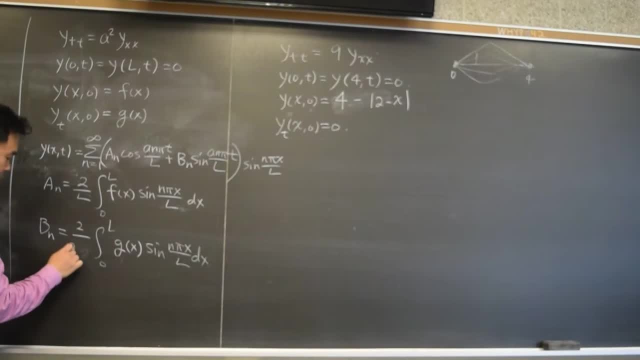 n pi. oh okay, so I right, right, right n pi. oh okay, so I right, right, right, 2 over a n times pi. thank you, that's all 2 over a n times pi. thank you, that's all 2 over a n times pi. thank you, that's all strong okay. 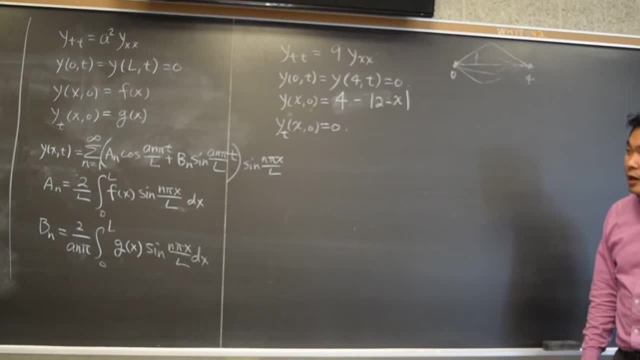 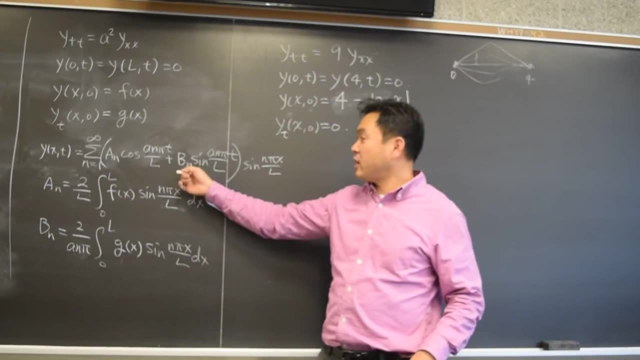 strong, okay, strong, okay, the same. no, no, a and B are different the same. no, no, a and B are different the same. no, no, a and B are different because when you do the matching of the, because when you do the matching of the, because when you do the matching of the coefficients to to get the B n, you have. 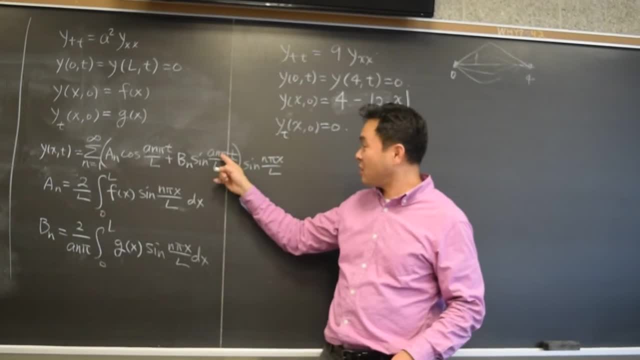 coefficients to to get the B n. you have coefficients to to get the B n. you have to match with the derivative and at some to match with the derivative and at some to match with the derivative. and at some point when you differentiate this a and point when you differentiate this a and. 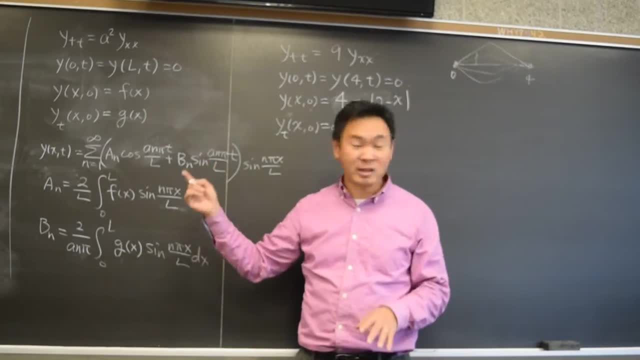 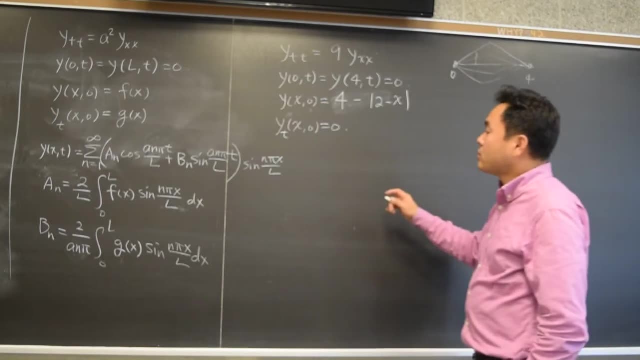 point, when you differentiate: this a and pipe pops out. and this, this L, also pipe pops out. and this, this L, also pipe pops out. and this, this L also pops out. they can't set in the result, alright, so let's, let's do the solution. alright, so, let's, let's do the solution. 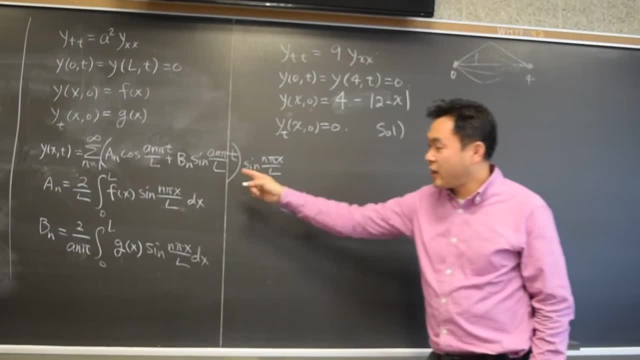 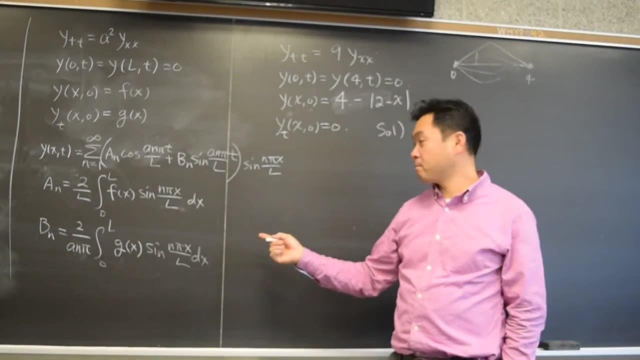 alright, so let's let's do the solution now. the solution is: you calculate a. and now the solution is: you calculate a. and now the solution is: you calculate a and calculate B n 1 under a 0, which one? okay. calculate B n 1 under a 0, which one? okay. 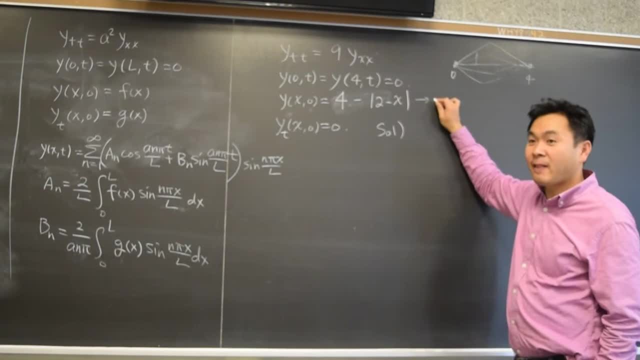 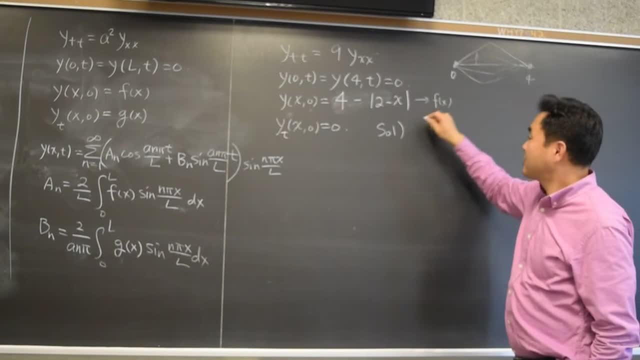 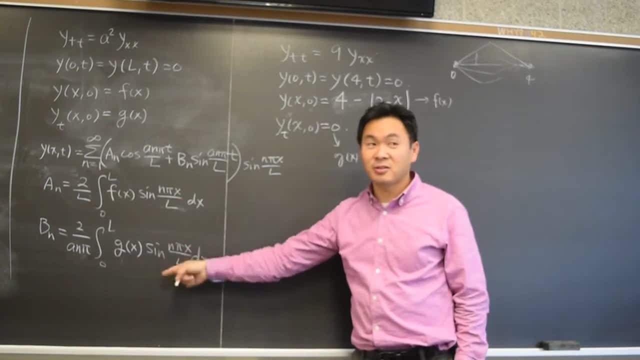 FX. and this one is yeah, GX, if you can FX. and this one is yeah, GX, if you can compare it to that one. okay, so which one compare it to that one? okay, so which one compare it to that one? okay, so which one is here? yeah, this one, GX, is here. so this. 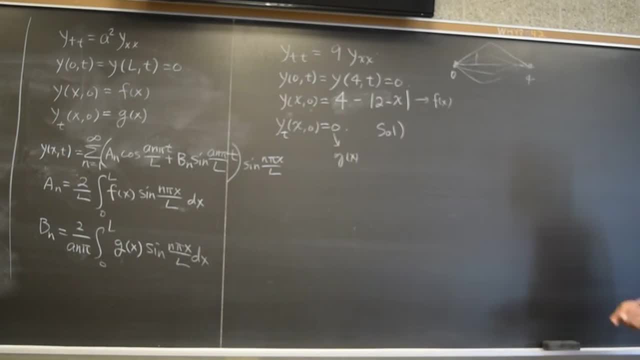 is here. yeah, this one GX is here. so this is here. yeah, this one GX is here. so this interval will give you zero. okay, so that interval will give you zero. okay, so that interval will give you zero, okay. so that means you just have to find a and once. 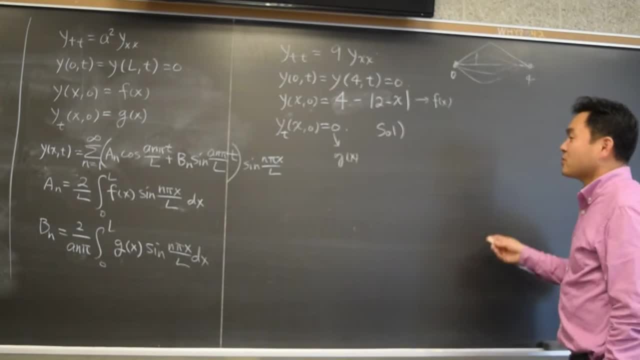 means you just have to find a, and once means you just have to find a, and once you find a and you plug it in here. and you find a, and you plug it in here, and you find a and you plug it in here, and then that's it. so that's, let's do that. 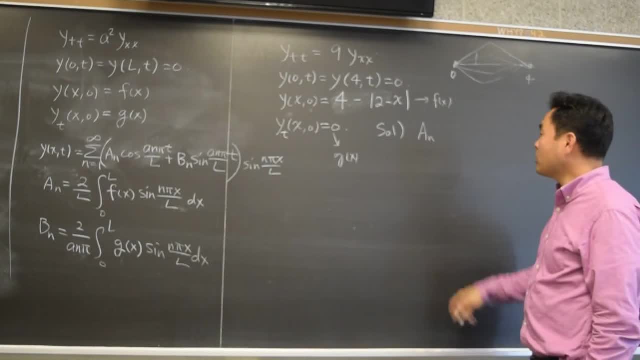 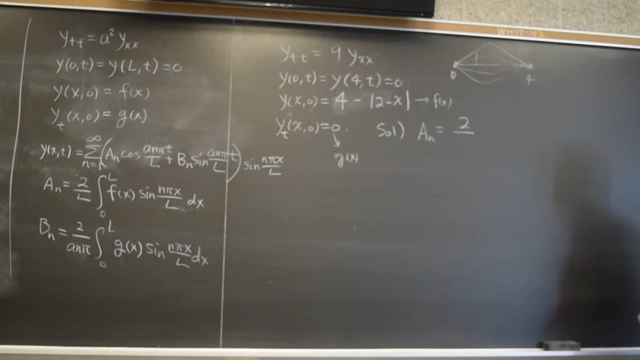 then that's it, so that's. let's do that, then that's it, so that's: let's do that. now we have to find a n which is you. now we have to find a n which is you. now we have to find a n which is you. take 2 over L. what is L here? 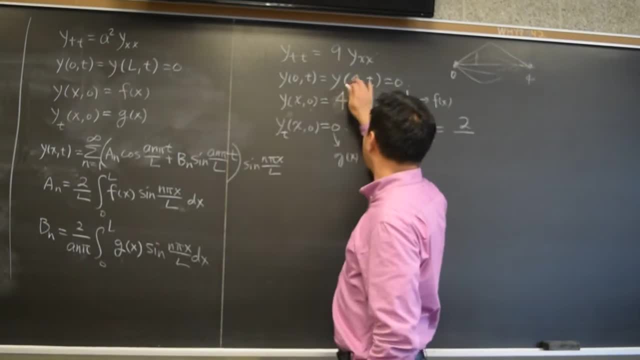 L is 4 L is the length of the. the L is 4 L is the length of the. the L is 4 L is the length of the. the streaming. if you look at here and you streaming, if you look at here and you streaming, if you look at here and you look at here, there's there's an L here. 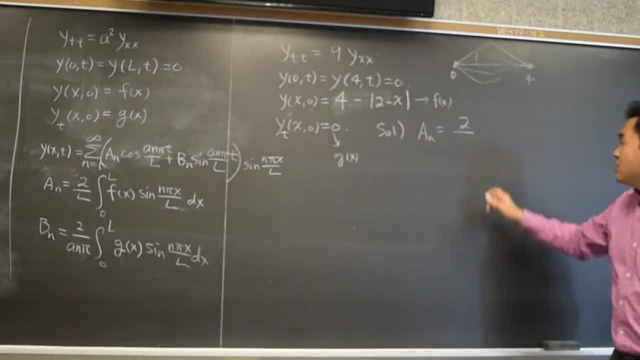 look at here, there's there's an L here. look at here, there's there's an L here. there's four there, so that must mean there's four there. so that must mean there's four there. so that must mean that L is 4. I mean just just by. 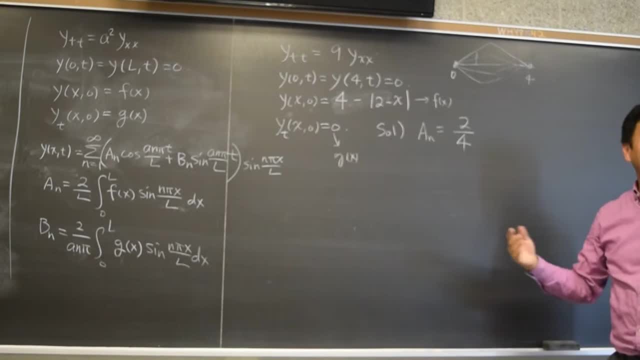 that L is 4, I mean just just by that L is 4, I mean just just by matching each, each equation carefully, matching each, each equation carefully, matching each, each equation carefully. you can figure out what L is, but you can. you can figure out what L is, but you can. 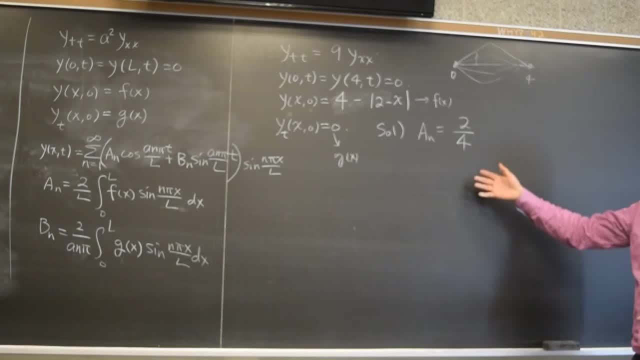 you can figure out what L is, but you can figure out what FX is and GX is. and figure out what FX is and GX is. and figure out what FX is and GX is and after after that, all you have to do is after. after that, all you have to do is: 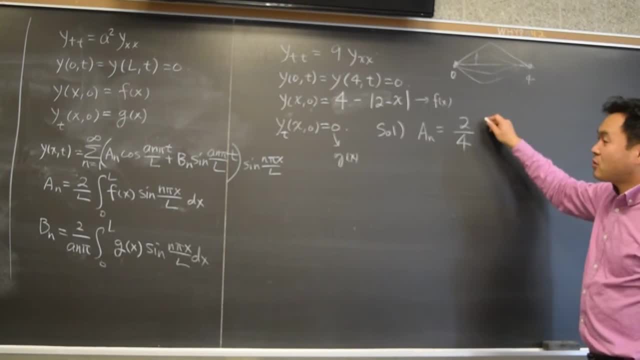 after after that, all you have to do is just just calculate, that's it. so you just just calculate that's it. so you just just calculate, that's it. so you have this 2 over 4 and then integral 0, have this 2 over 4 and then integral 0. 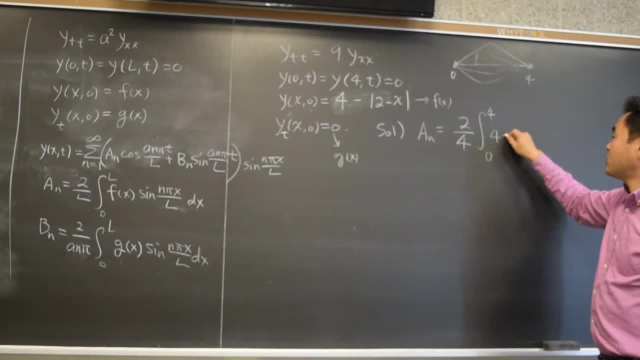 have this 2 over 4, and then integral 0 to 4 FX is 4 minus epsilon del your 2 to 4. FX is 4 minus epsilon del your 2 to 4. FX is 4 minus epsilon del your 2 minus X. and then you have to multiply by: 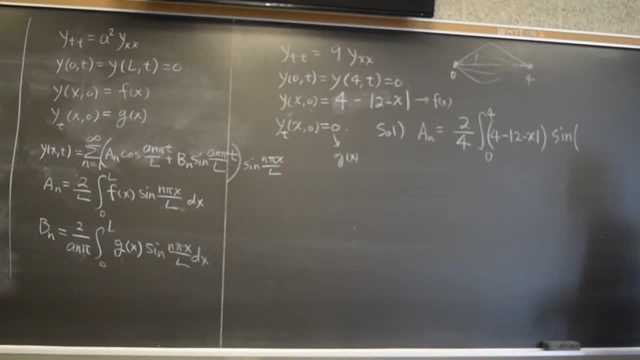 minus X, and then you have to multiply by minus X, and then you have to multiply by sine of what, and I X over 4, so that's sine of what, and I X over 4, so that's sine of what, and I X over 4, so that's what you have to do, and pi X over 4. 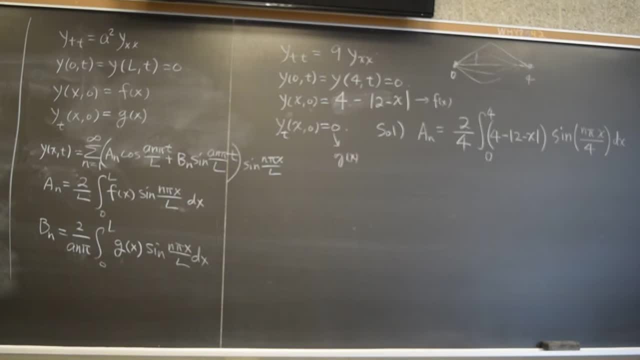 what you have to do and pi X over 4 what you have to do and pi X over 4 sounds easy, right. sounds easy, right. sounds easy, right. The only trouble is that now you need the integral. that's split into two parts because of this epsilon value. 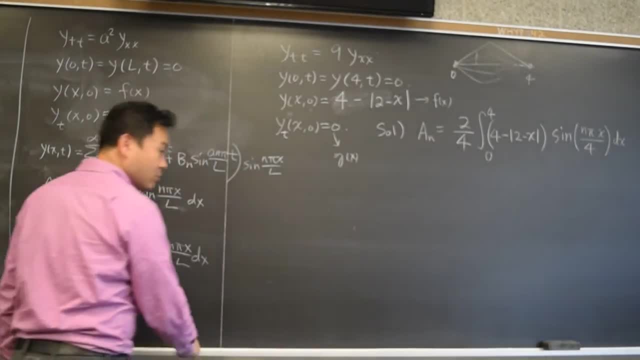 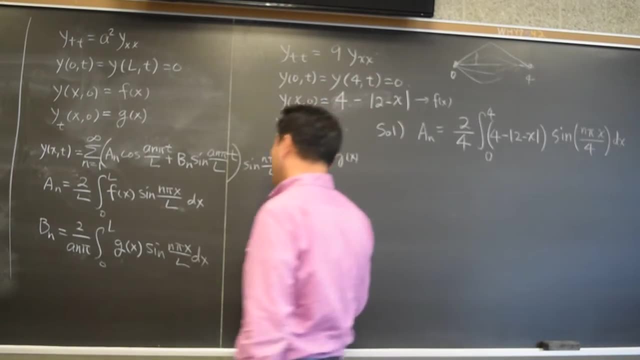 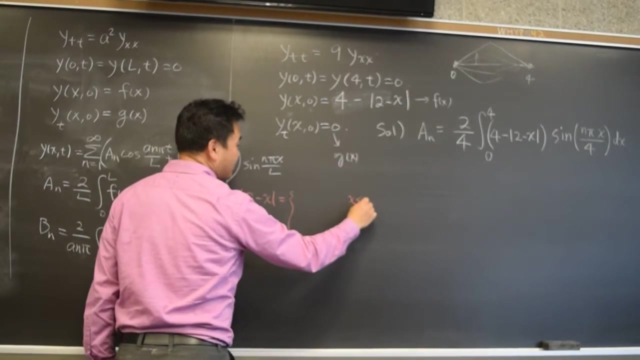 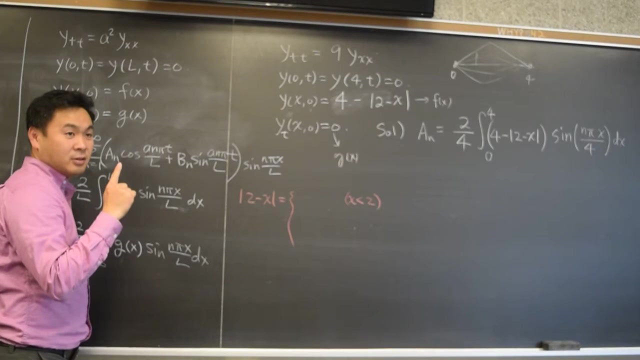 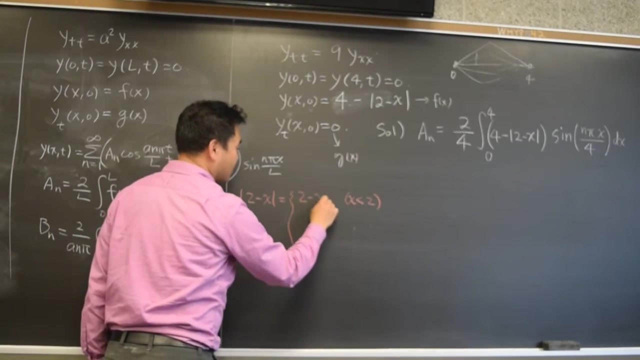 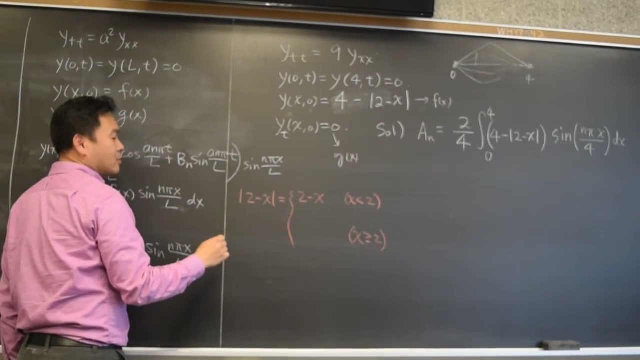 So what is 2 minus x epsilon value? What is 2 minus x epsilon value? So if x is less than 2, 2 minus x is positive or negative. Positive, So what does the epsilon value do? Nothing If x is bigger than 2, what happens? 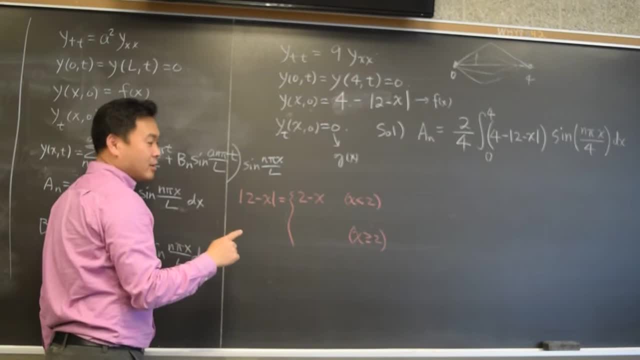 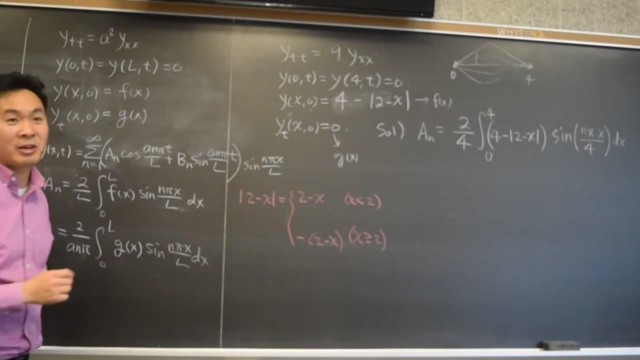 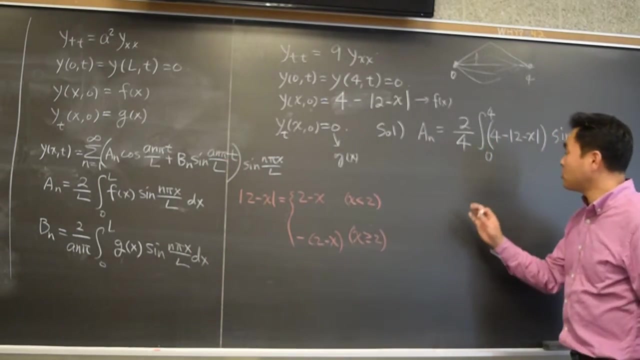 This will be negative. therefore It makes it positive. How do you make a negative value positive? You put a negative in front that will make it positive. So that's what 2 minus x is and therefore, when you do this integral, you should split. 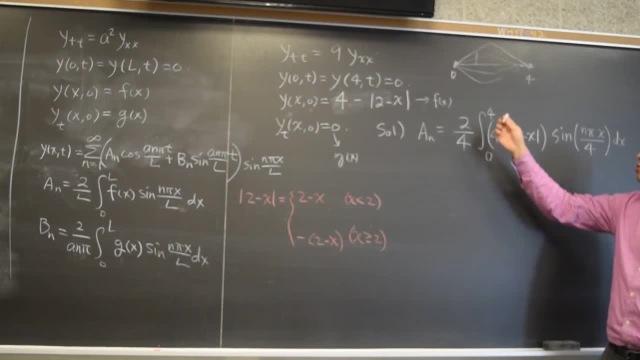 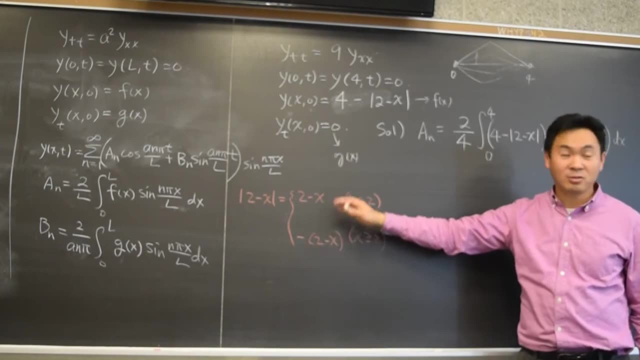 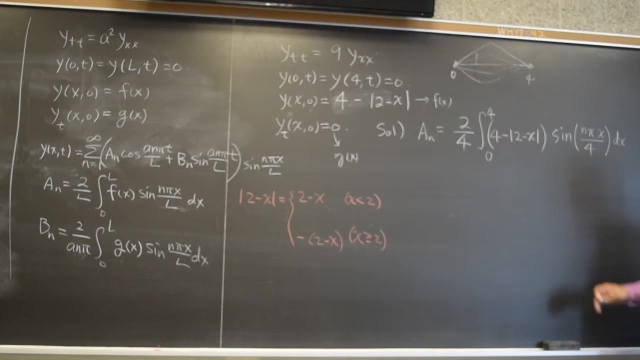 the integral from 0 to 2 and 2 to 4, and once you have that, and then you will need to use these two different definitions of the epsilon value of 2 minus x, and afterwards you should help it. Okay, Let's go a little bit more. 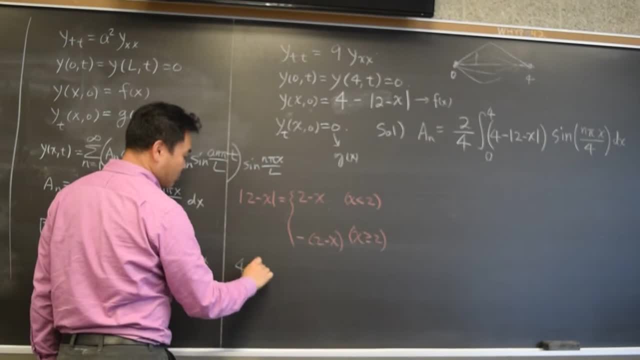 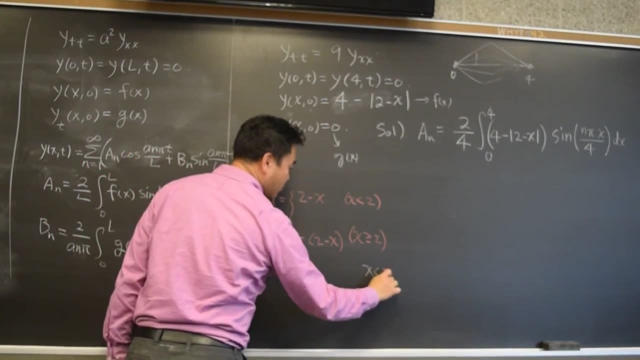 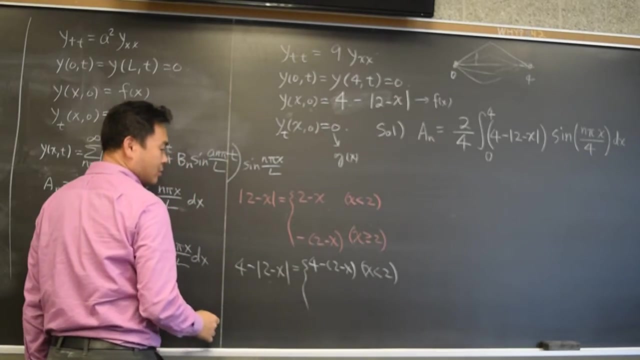 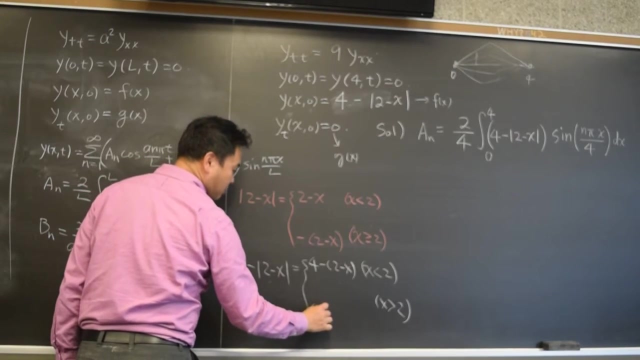 What is 4 minus 2 minus x? then 4 minus 2 minus x is when x is less than 2, this will be 4, it says 4 minus 2 minus x. It doesn't change. But if x is bigger than 2, then it will be 4 minus negative 2, so it will be 4 plus 2. 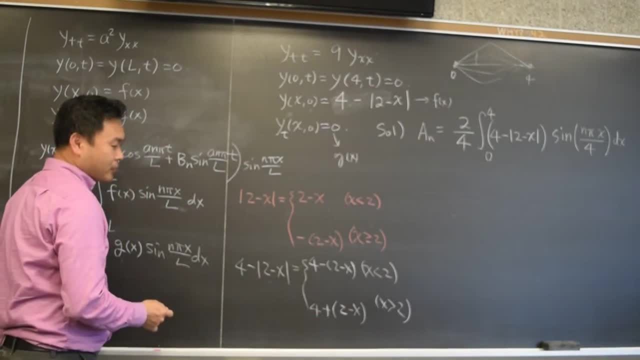 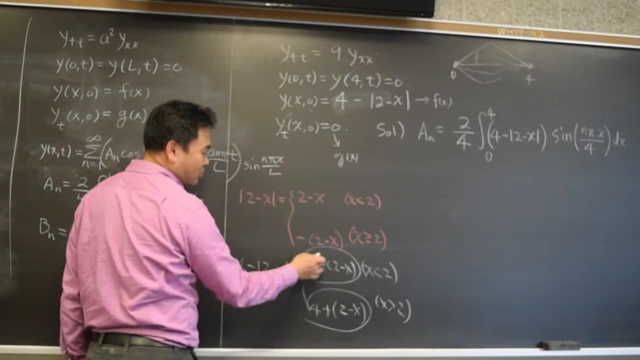 minus x. Okay, So it will be these two functions, and of course you should simplify further, because 4 minus 2 is 2, so this will be 2 plus x, whereas this will be 6 minus x. so that's what we will use. 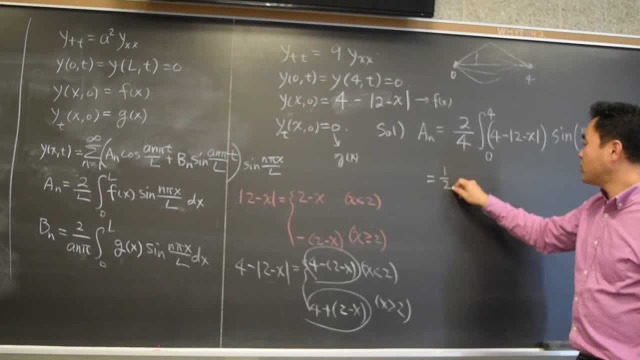 Okay, So integrate 1 half. first one is 0 to 2. of this one from 0 to 2, we follow this one, which is 4 minus 2 is 2.. So it's 2 plus x Okay. 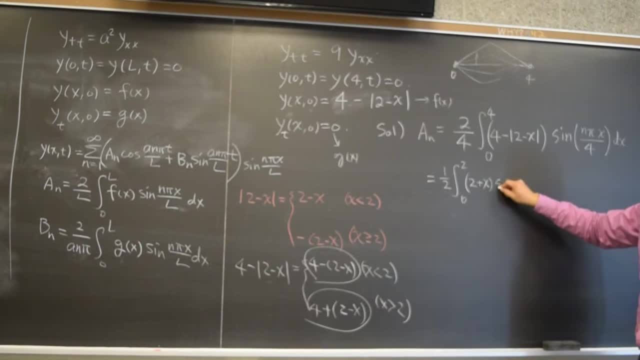 So 2 plus x times sine of n pi over 4x dx, and then plus- I'll just put it here- plus 1 half integral from 0 to 2, this one is 6 minus x, right? so you put 6 minus x sine. 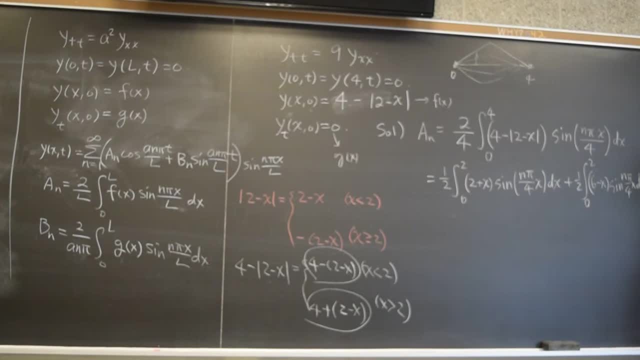 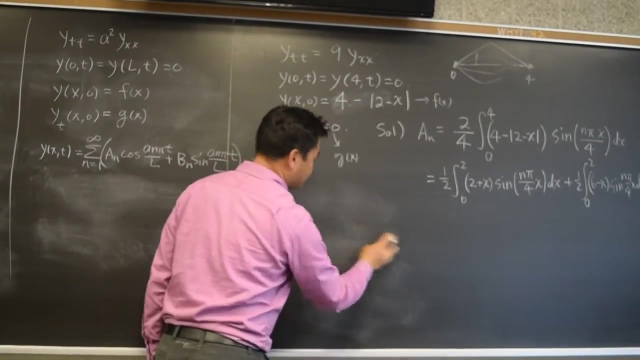 n, pi over 4.. Okay, So this is the integral of x, dx. Okay, Each of these should be computed using using a tabular integration. Let me erase this part because I don't need this anymore. Let me compute it here. 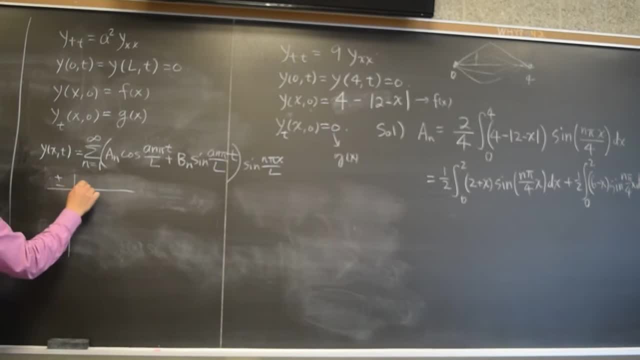 So for the first integral you need plus minus D integral and you have 2 plus x and then sine n pi over 4x. Now, if you differentiate this, it's 1.. If you differentiate this, it's 0.. 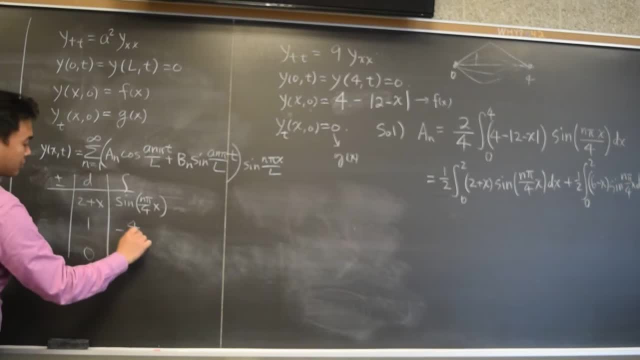 If you integrate this, that's negative: 4 over n pi cosine n pi over 4x And integrating again it's negative. 16 over n square pi squared cosine no sine n pi over 4x and plus minus plus. 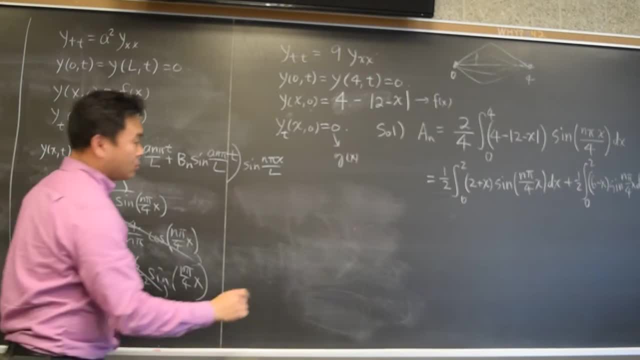 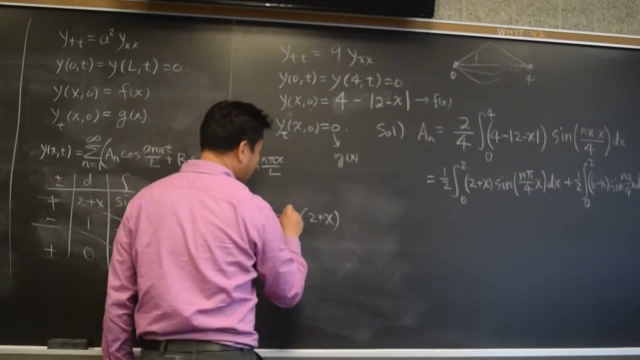 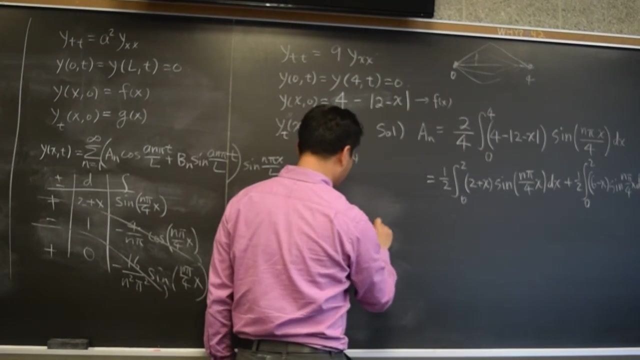 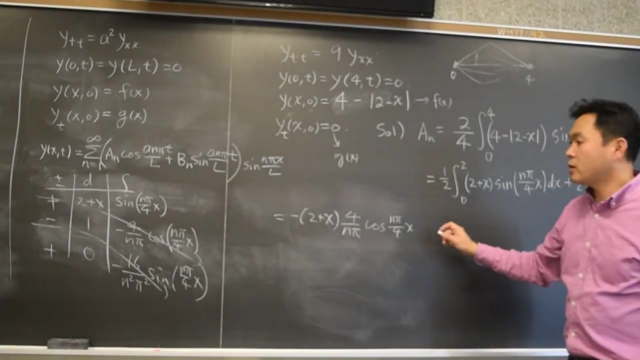 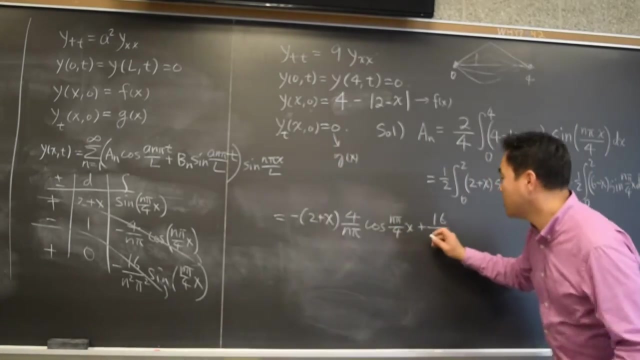 And doing that and that will give you the following integral: It will be 2 plus x multiplied by negative: 4 over n pi, 4 over n pi, cosine, n pi over 4x, And then negative negative will be positive, so it will be plus 16 over n squared pi squared. 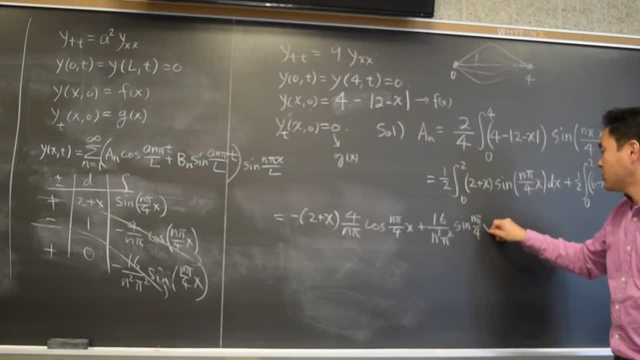 sine n, pi over 4x, And then you will have to plug in x, And then you will have to plug in the endpoints 2 and 0.. That's for the first one. For the second one, let's see. I guess we can skip a little bit. 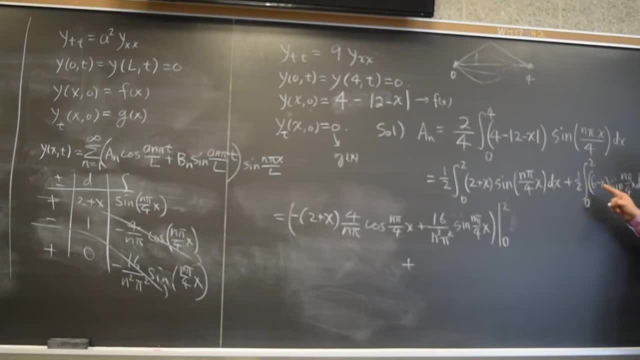 Because really the only thing that's different from this one to that one is, instead of 2 plus x, you have 6 minus x. That's the only difference, right, And the next it will be 6 minus x and then negative 1.. 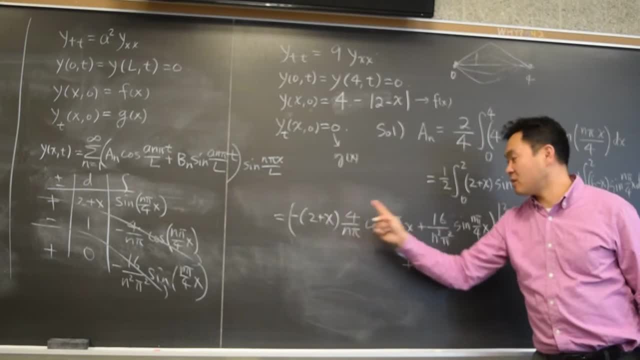 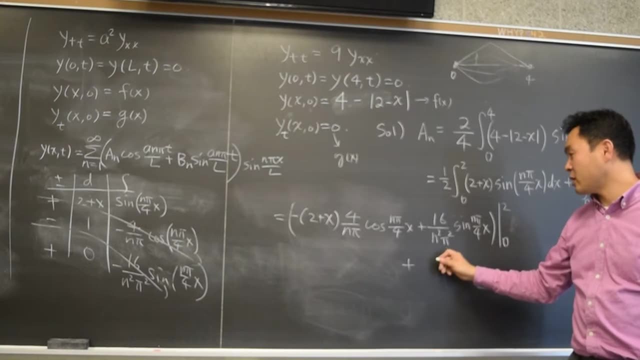 So there's this and positive 1 here, But I will replace this by 6 minus x and this will be negative 1 in front. So for the second one, you will be getting negative 6 minus x, 4 over n pi. cosine n pi. 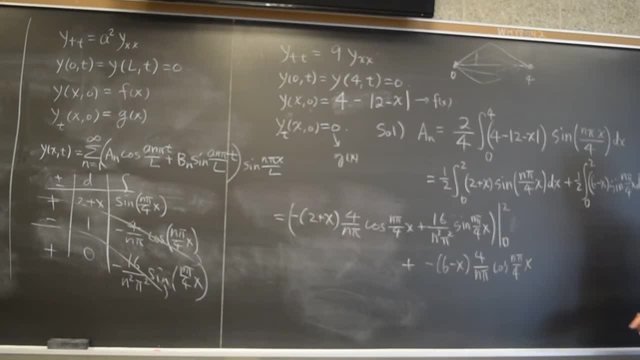 over 4x, And for the second one you will be minus 16 n squared pi squared sine n pi over 4x, And for this one you will be plugging in 4 and 2.. Sorry for skipping this, just to save time. 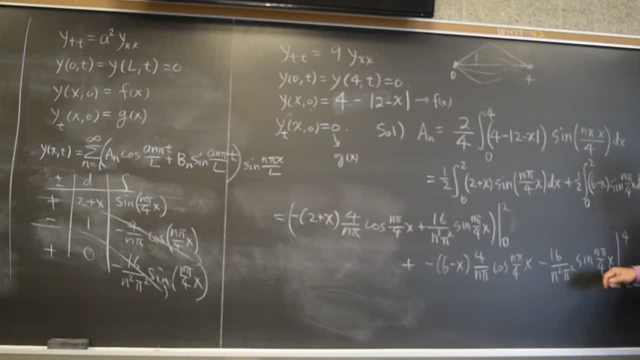 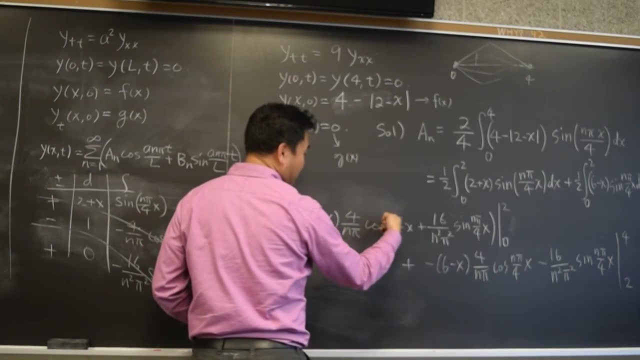 But if you want to check, you can do the same tabular again. You'll find out that I did this right. OK, All right, Now let's plug in 2.. If you plug in 2 here, you get 4, cosine 2, n, pi over 4.. 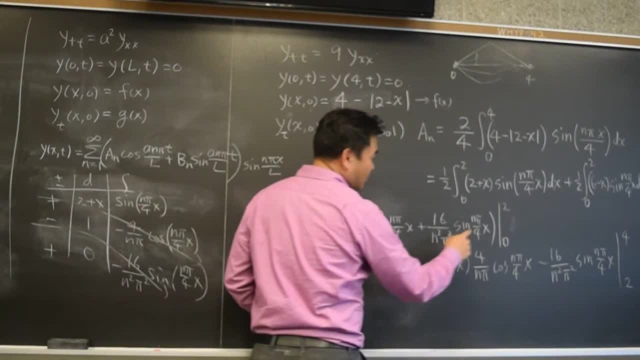 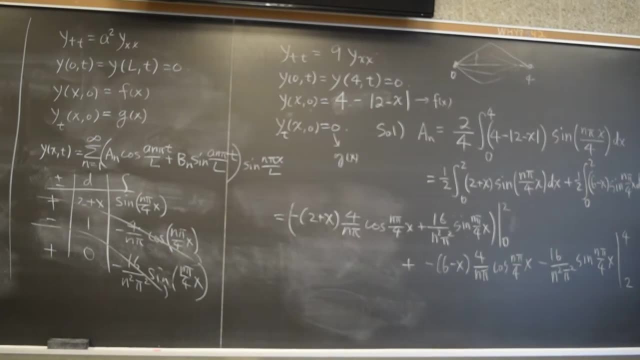 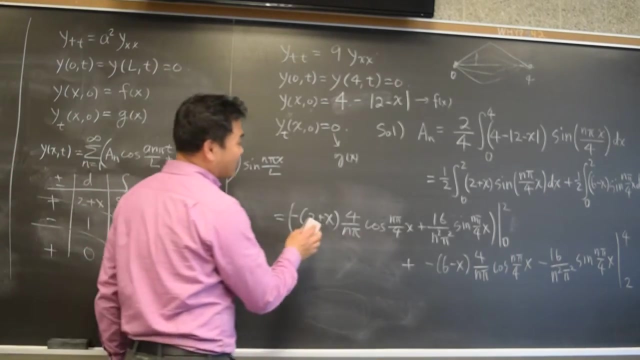 OK, That's going to be causing some trouble here. This will also give you something. Oh, it's a mess. It's very, very tough, Much more involved than what I anticipated. OK, All right, I don't have any more choice but then to delete everything. 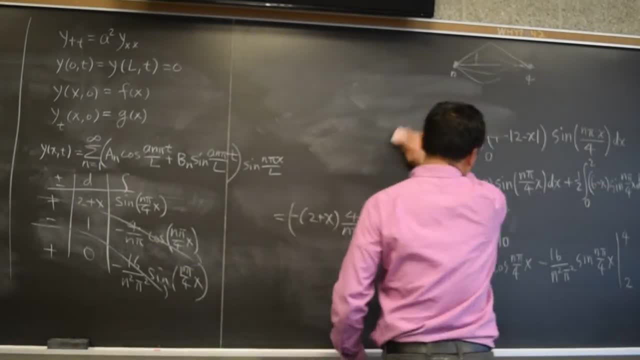 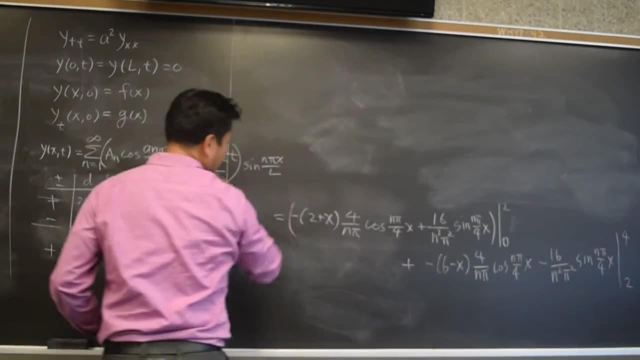 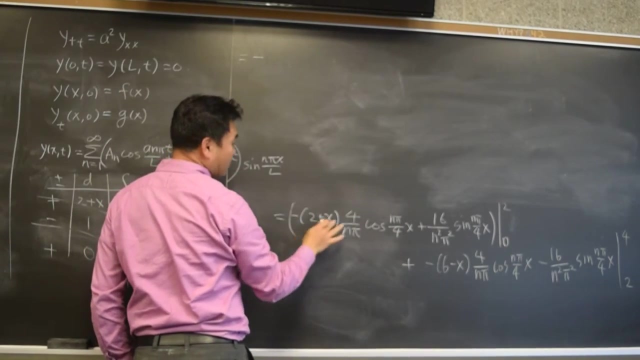 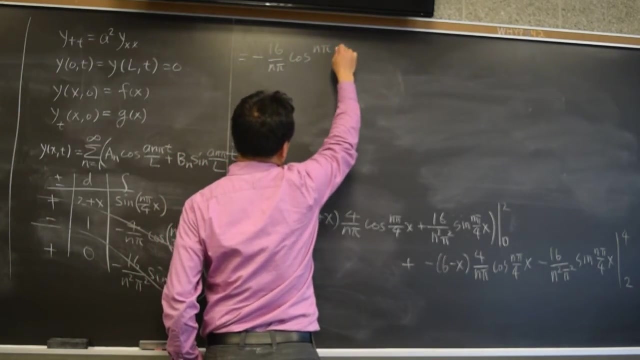 I'll just erase everything and start writing on top. OK, So let's start writing one by one. First, when you plug in 2, it's negative 4 times 4.. So that's 16 over n pi. cosine n pi. 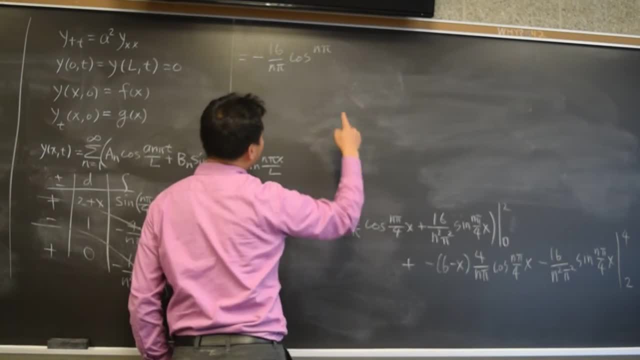 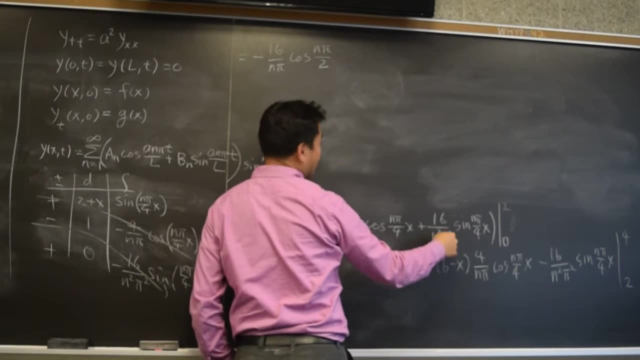 And if you plug in 2 here, 2 and 4 cancels right, So you get 2.. And then again, if you plug in 2 here, 2 and 4 cancels and you get sine n pi over 2.. 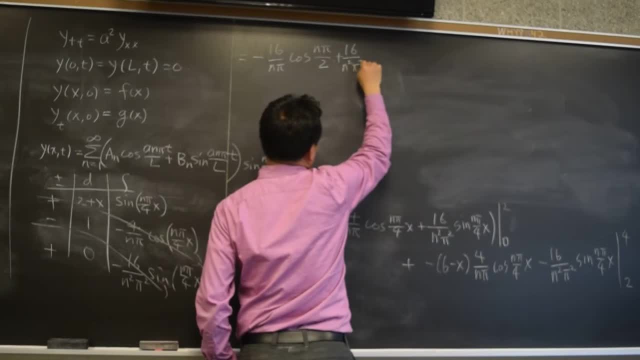 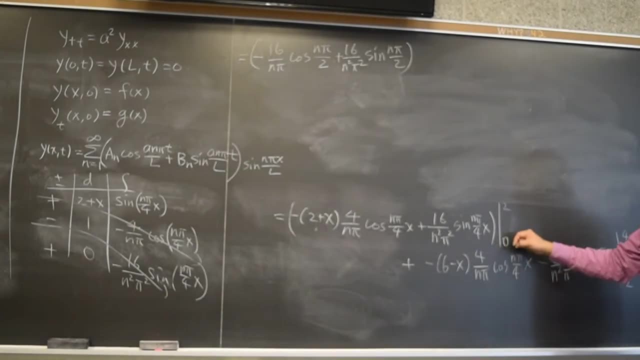 So you get plus 16 over n squared pi, squared sine n pi over 2.. So that's what you get if you plug in 2.. Now, when you plug in 0, cosine 0 is 1 and sine 0 is 0.. 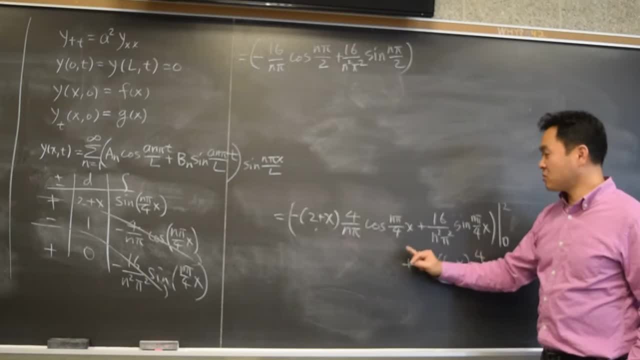 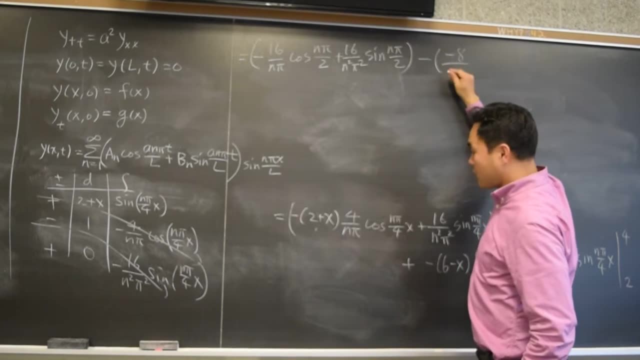 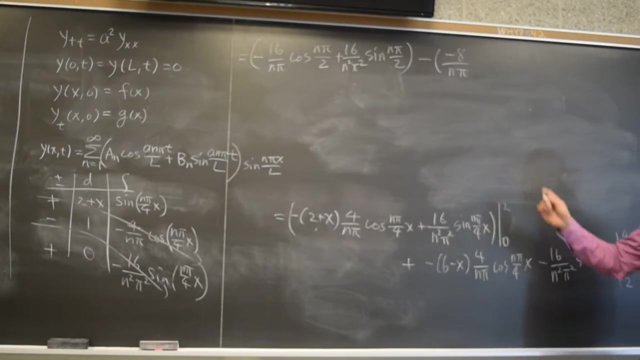 So that one's gone. so that's good, This one survives and we have to take care of it. OK, If I plug in 0, it's negative 8 over n pi and cosine of 0 is 1, so that's it right. 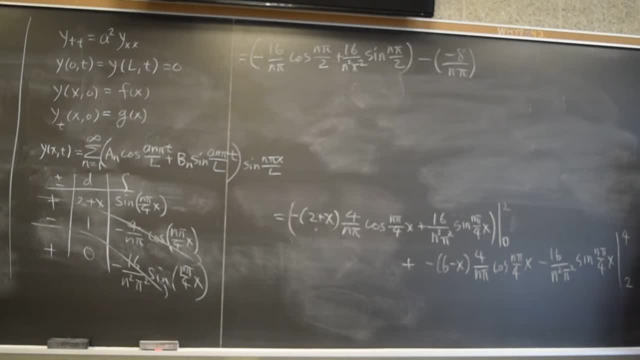 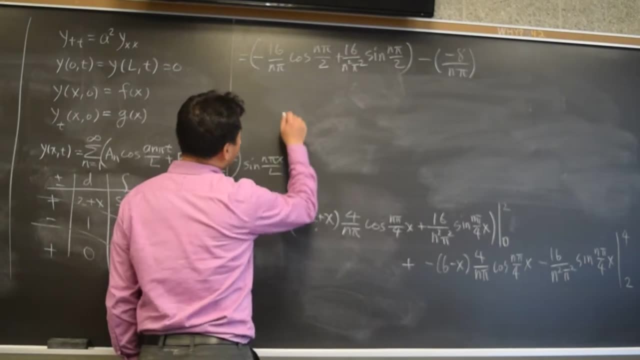 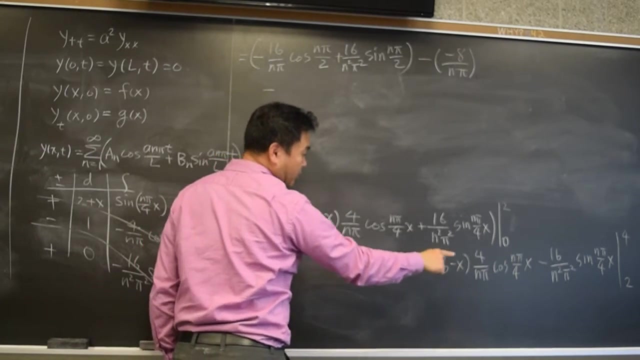 So that's what you get from the first integral. OK. Now in the second integral it's Negative. Plugging in 4 gives you cosine n, pi, which is negative 1 to the nth power right, And if you plug in 4, it's negative 8.. 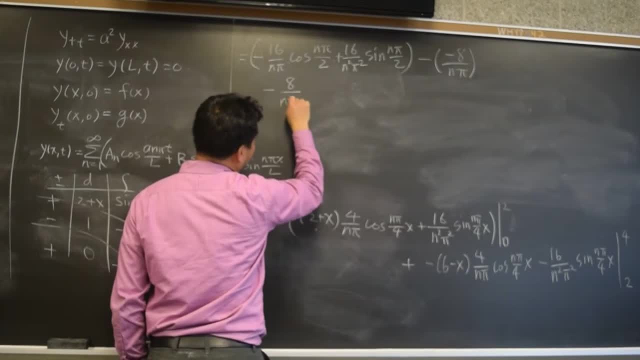 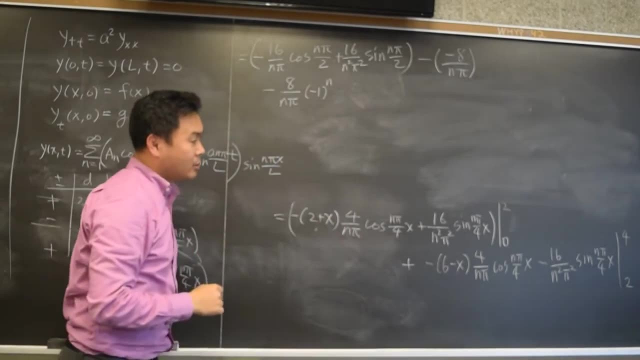 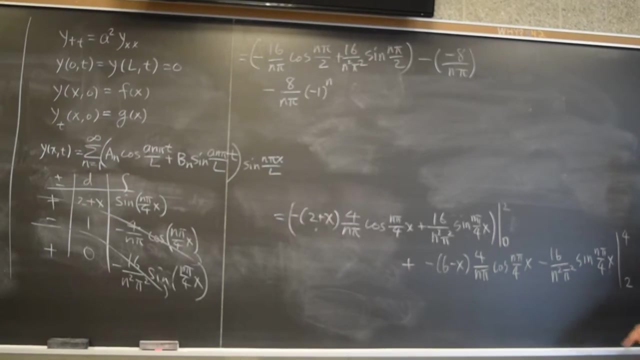 So it's negative 8 over n pi, And this is negative 1 to the nth power, because you get cosine n pi, And plugging in 4 here gives you sine n pi, which is 0.. So that's, That's all you get, OK. 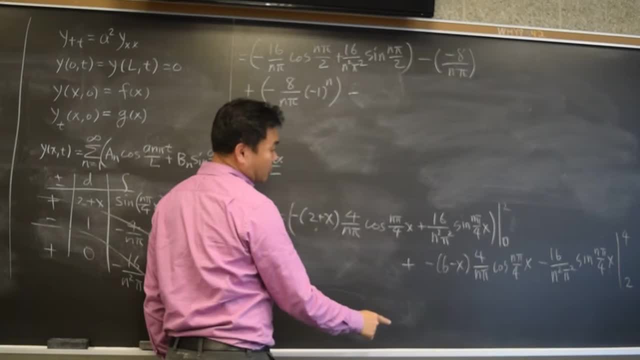 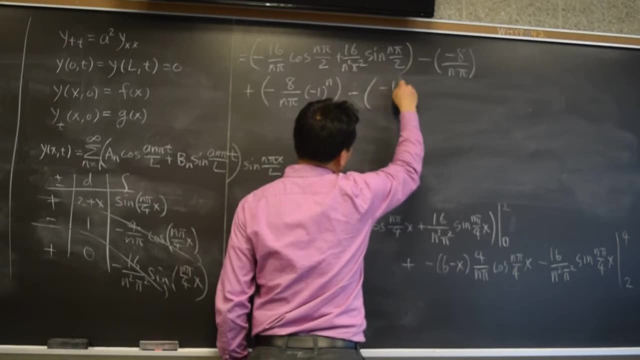 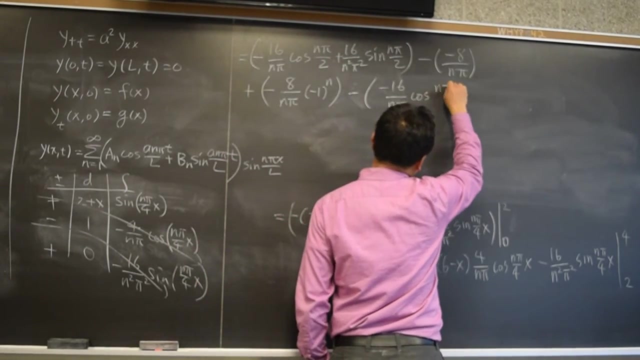 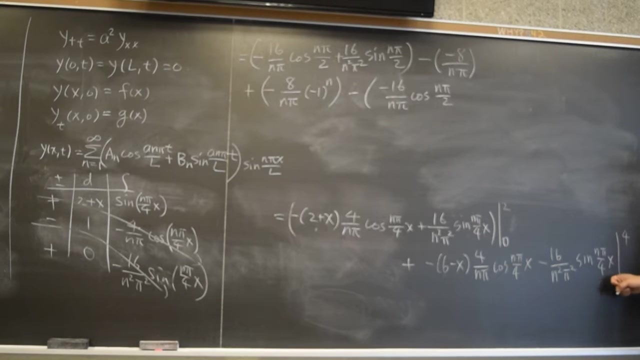 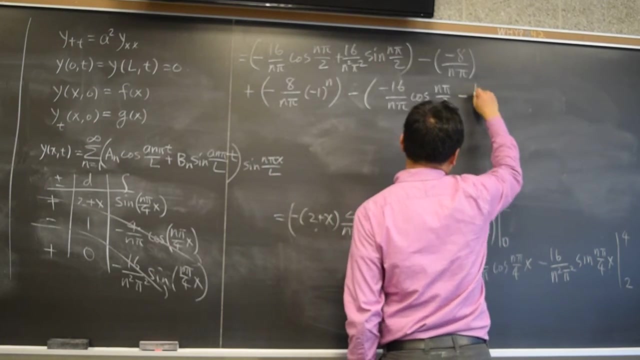 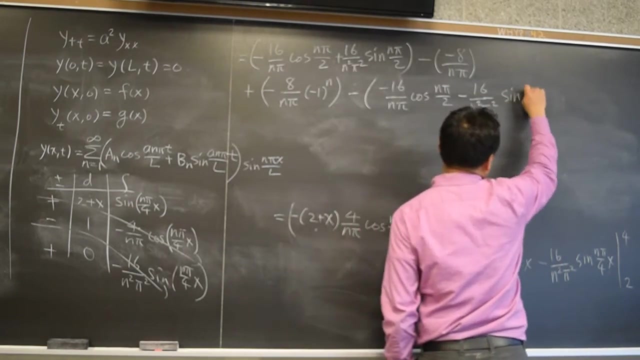 And then finally, when you plug in 2, this becomes 6 minus 2, which is 4.. 4 times 4 is 16, so negative 16 over n pi Cosine n pi over 2.. OK, And then when you plug in here, you get negative 16 over n squared pi, squared sine, n pi over 2.. 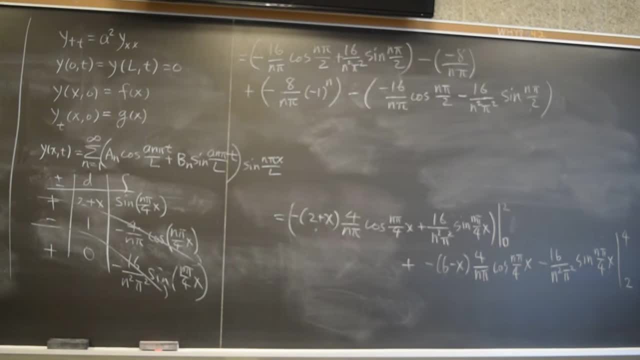 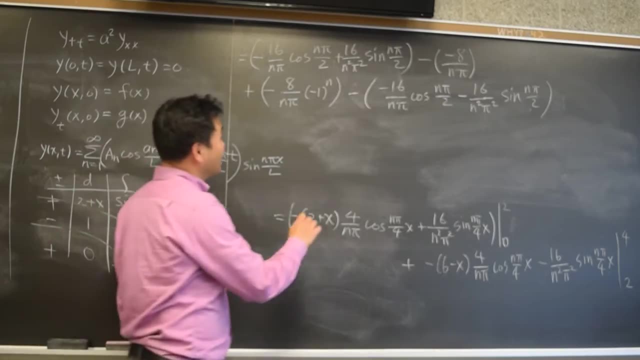 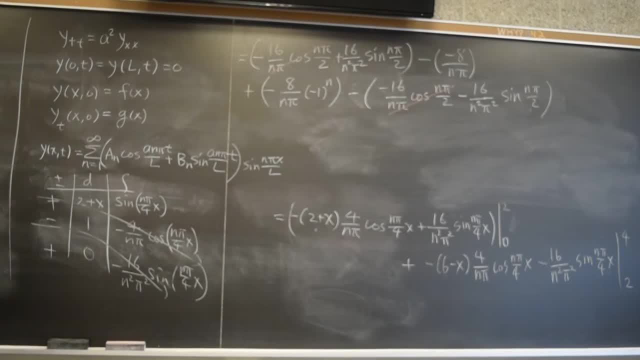 Minus minus is plus, so they double. All right, So let's write that down again. OK, All right. So still a good thing is that this and that is the same. So if we factor these two out, you get minus minus. 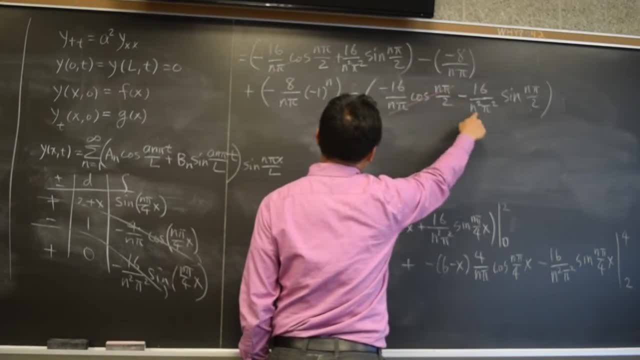 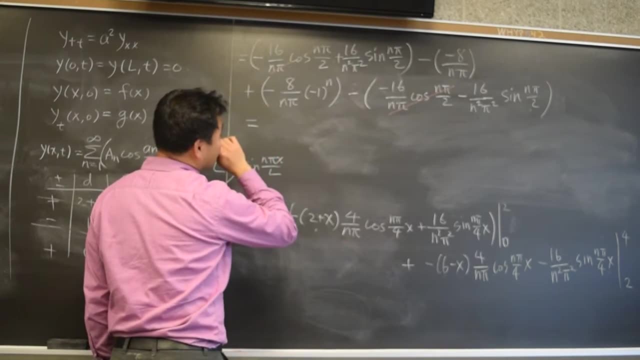 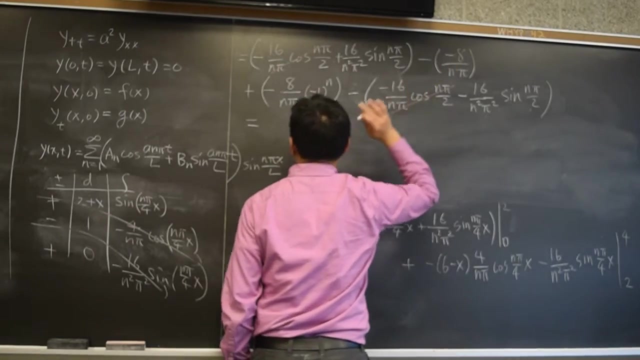 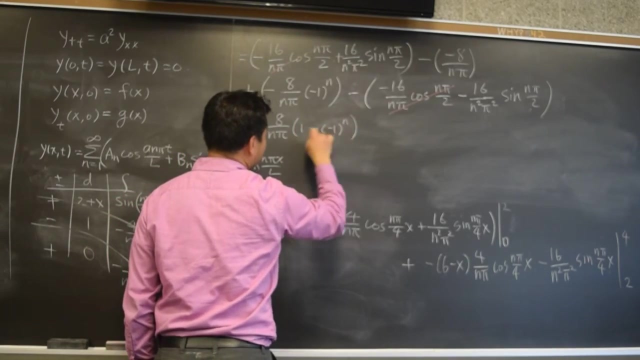 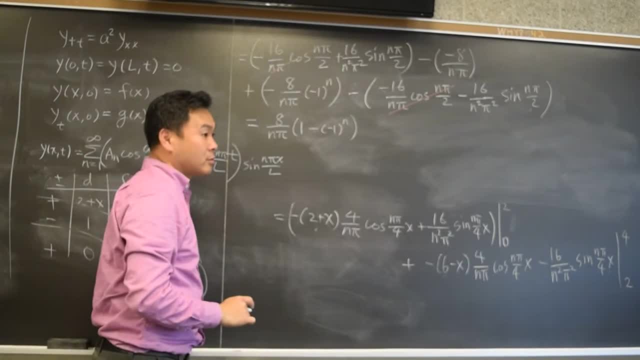 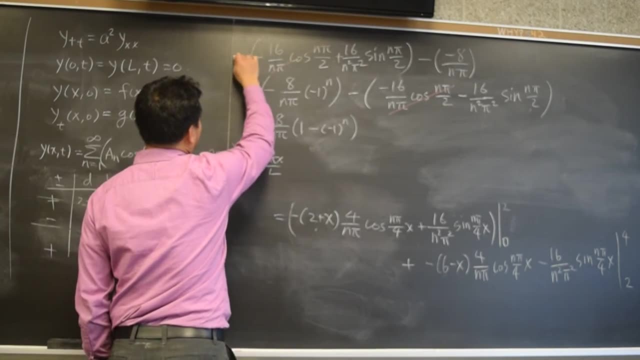 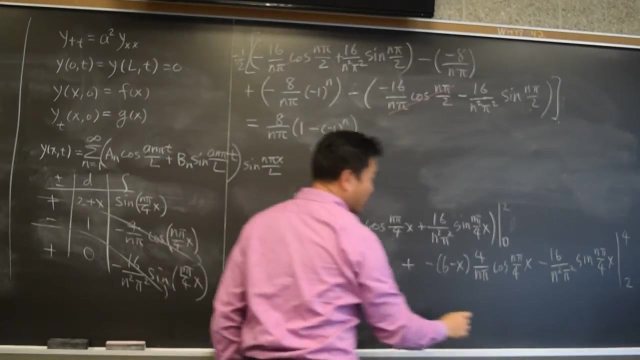 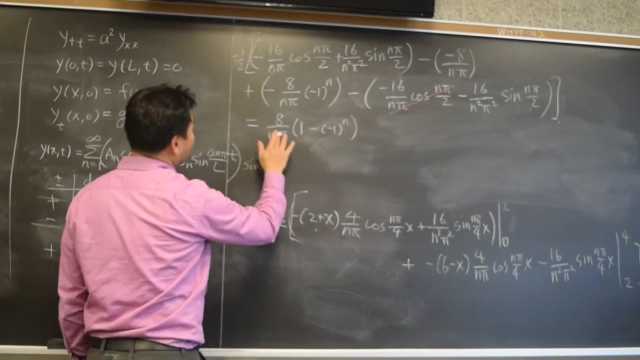 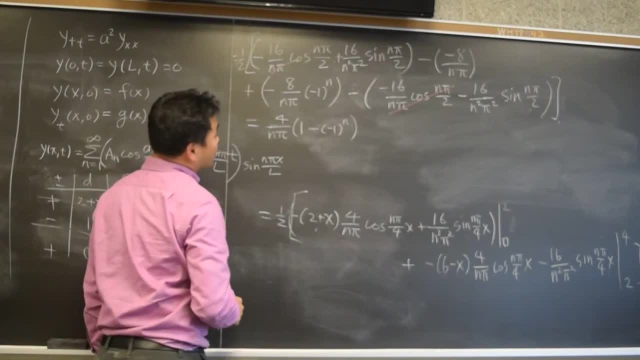 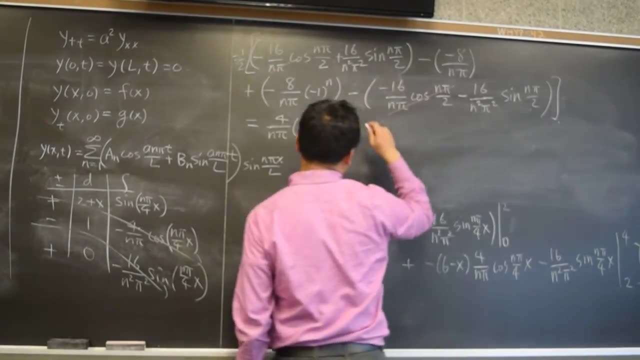 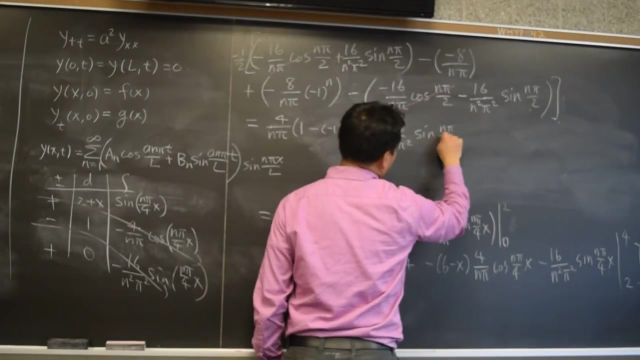 Yes, So So, Yes, Yes, You stay with me here. Okay, Yeah, Okay, Yeah, Yeah, Yeah, Okay, Yes, Yeah, You can go back, Ama, Okay, Yes, Yeah, Yes, Yes. 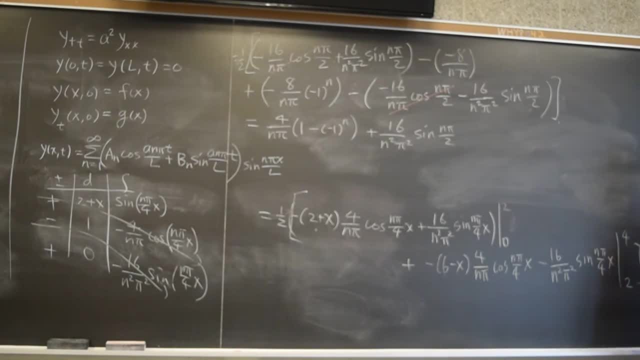 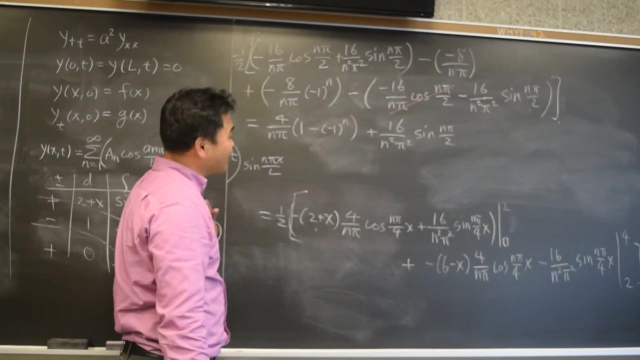 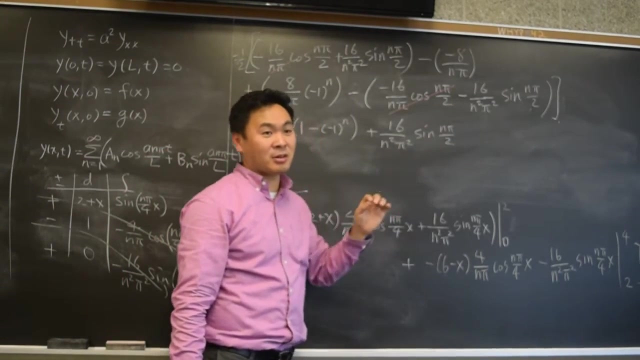 Yes, Yes, Yes. Now, this is somewhat. this is somewhat. it's not as what we like it to be, because sine n, pi over 2 is definitely a number that oscillates between what? 0, 1, 0, negative 1, 0. 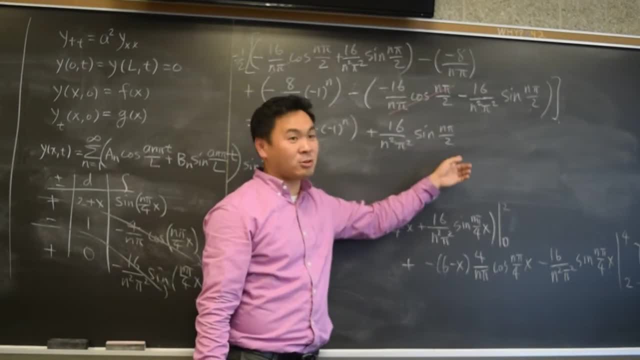 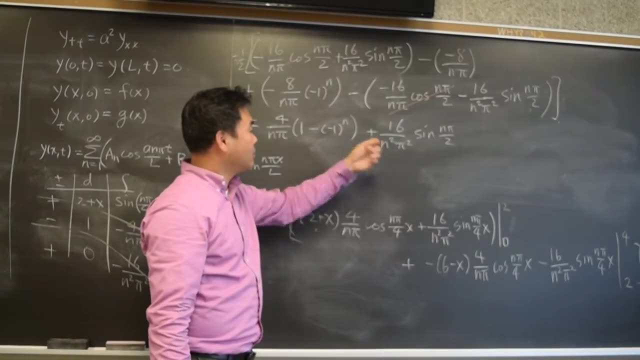 So when n is even, this will be 0.. When n is odd, it will be either a positive 1 or a negative 1, right. So that's what happens. What about this one? What happens if this is even? 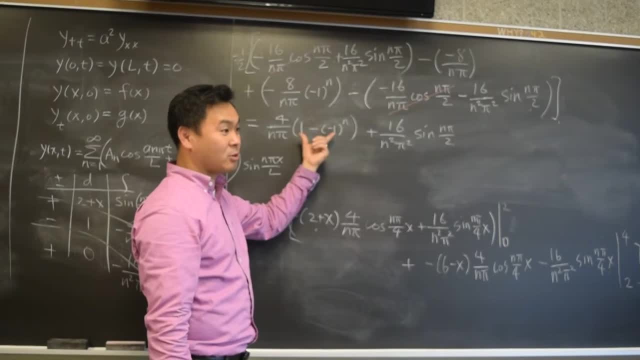 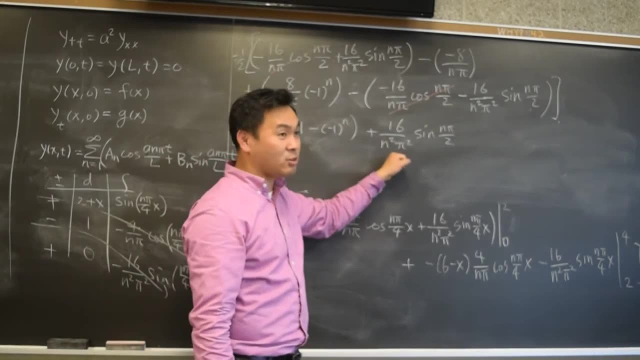 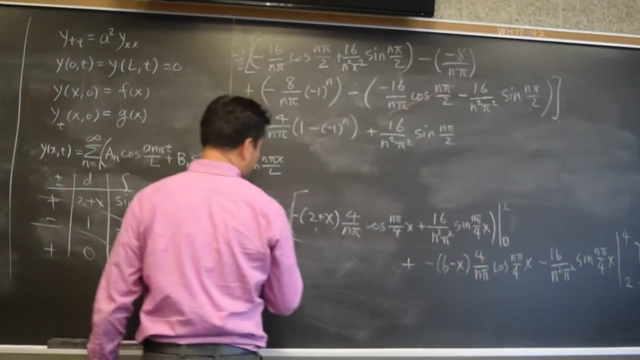 It'll be 0,, right, And it will only be. it will be 2 if n is odd, right? So you see that when n is even, they both give you 0.. So you should, you should. I'm trying to say something more about this, okay. 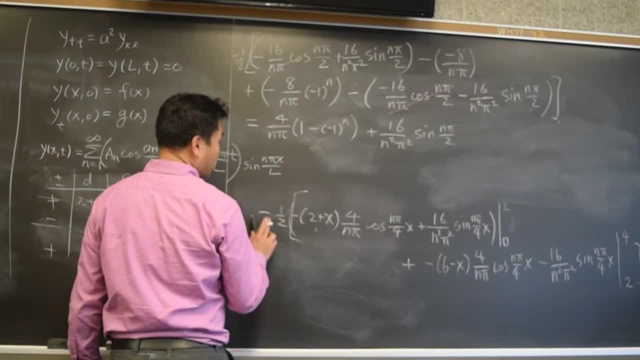 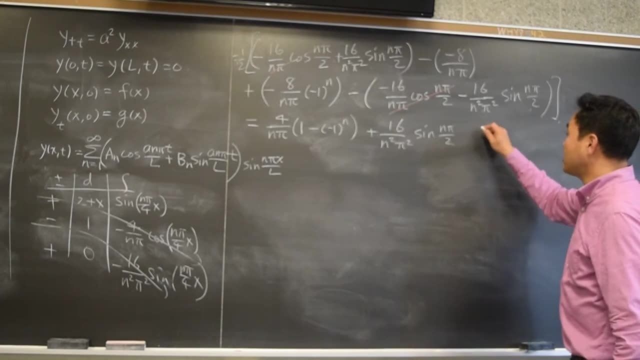 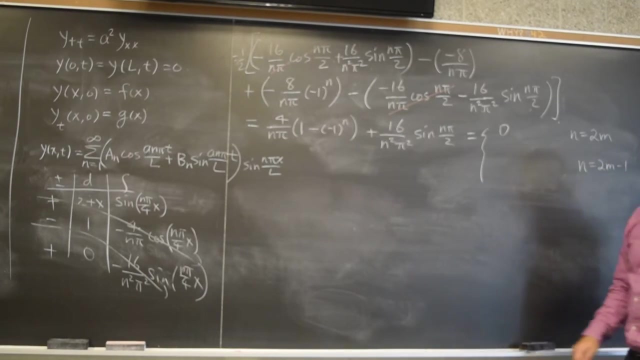 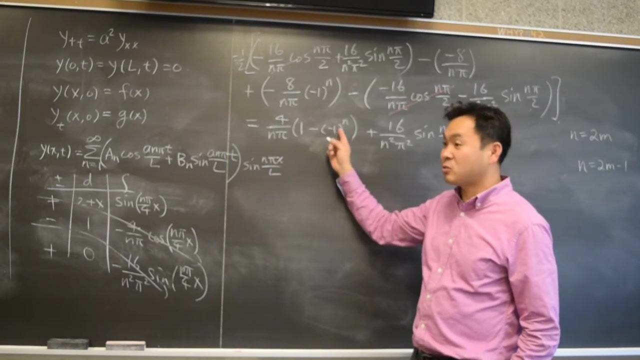 So we say that because this is 0, if n is 2m, it will give you 0,. okay, Now, if n is 2m minus 1, what's going to happen? This will double. Okay, This will be if it's odd power. it's negative 1, 1 minus negative. 1 is positive 2, 2 times. 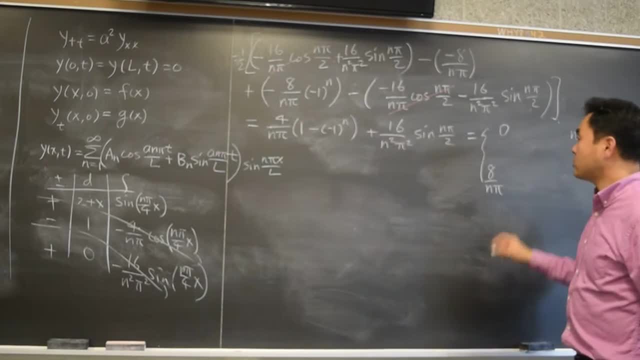 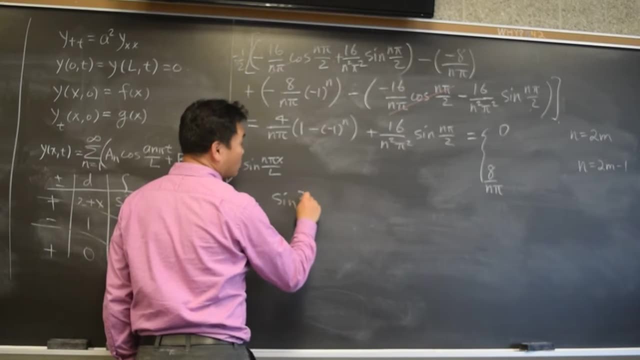 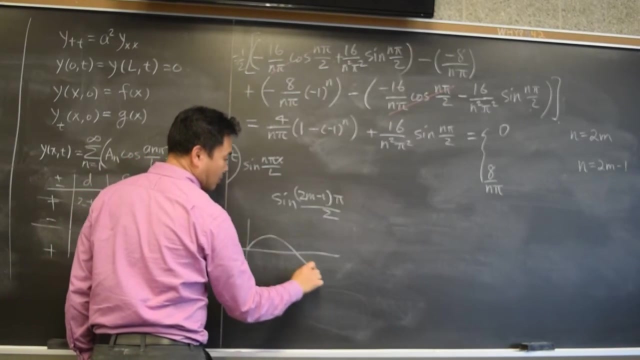 4 is 8 over n pi. That's what you get for the first one And this one. what is sine 2m minus 1 pi over 2?? Let's look at it. So here's pi over 2, here's 3 pi over 2.. 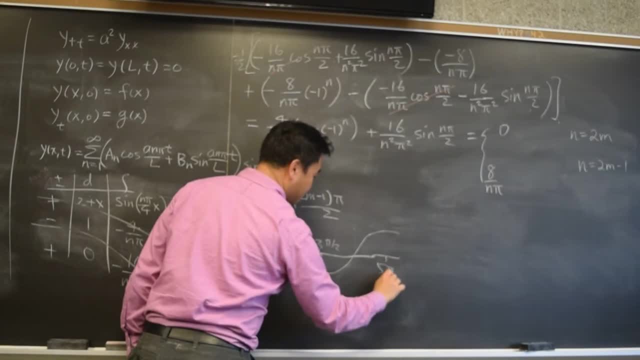 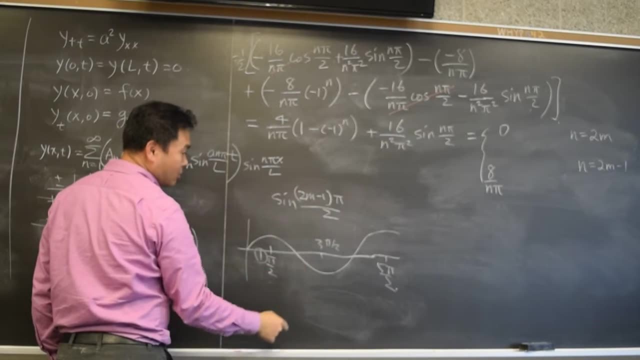 Here's 5 pi over 2.. Now 1 pi over 2, that corresponds to when m is 1.. If m is 1, it's 1 pi over 2.. When m is 2, if you plug in 2, you're 2 times 2 minus 1, that's that's negative 1.. 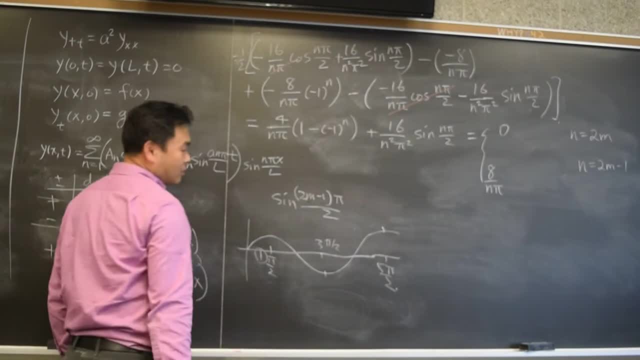 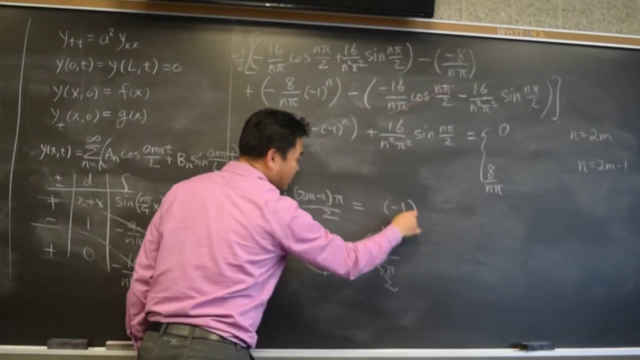 If m is 3, it's going to give you that, okay. So what do you see? If m is odd, you get 1, positive 1.. If m is even, you get negative 1.. So can you write this down as negative 1 to some power. 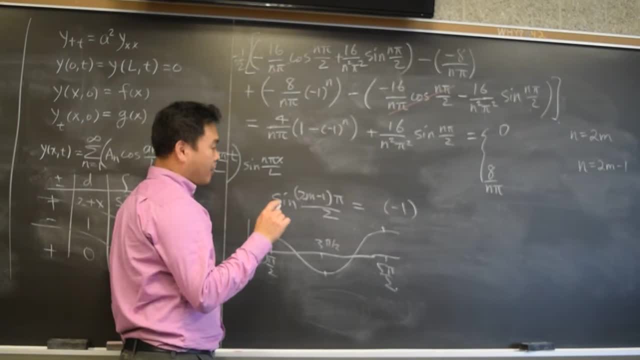 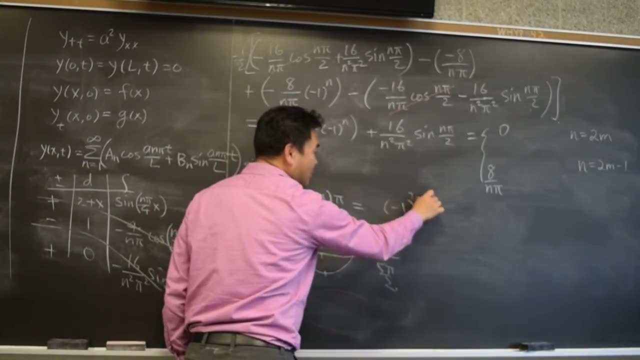 What 2m minus 1.. 2m? If it's 2m, that means it's already always positive. If it's 2m minus 1, that means you're taking odd power of negative 1, so it's always negative. 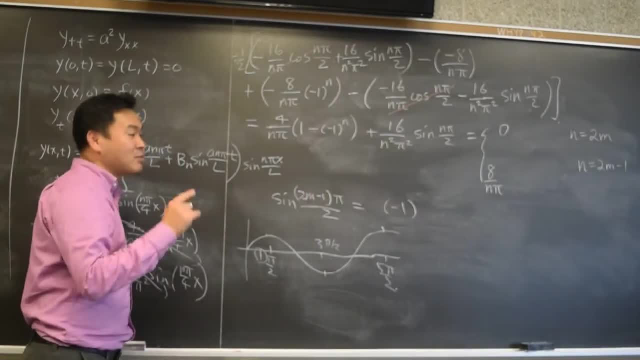 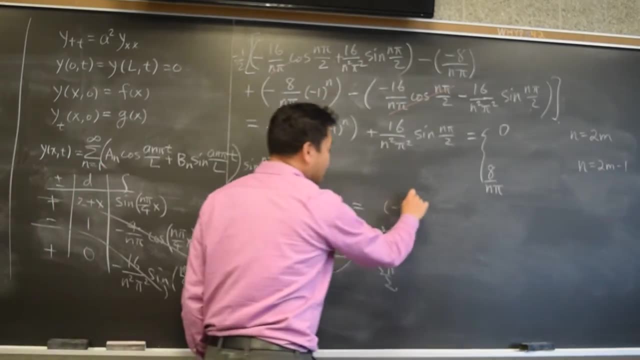 1. I want this to alternate whether m is positive, m is negative, m is odd or m is even Just n? n plus 1.. n plus 1.. That's what it is right, Can you see it? 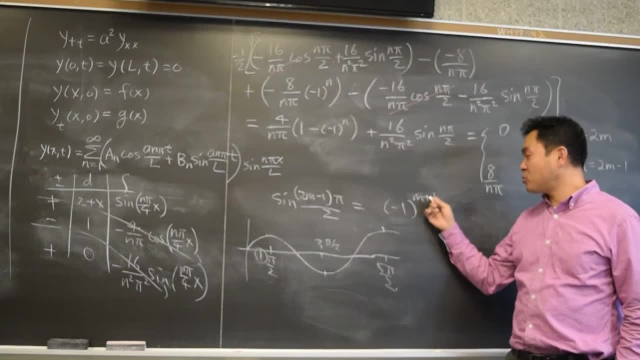 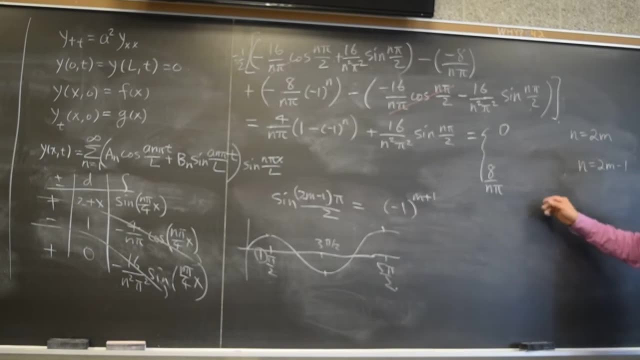 If m is 1,, 1 plus 1 is 2, negative 1 to the second power is 1, exactly as we have. Okay, So that's what we get. So we have, in that case, it's plus 16 over n squared pi squared over negative 1 to the. 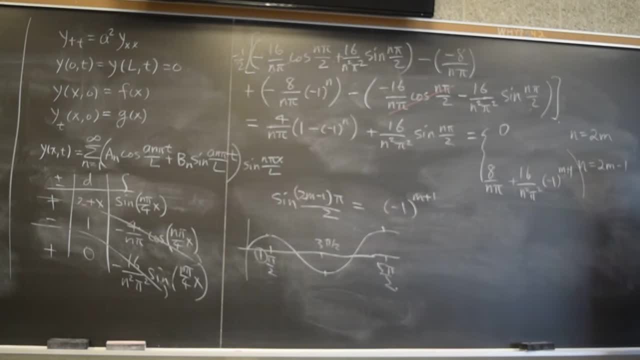 n plus 1.. Because we want to just replace all the n by 2m minus 1, we'll just rewrite this as 8 over 2m minus 1, pi plus 16, 2m minus 1 squared pi. squared negative 1 to the n plus 1.. 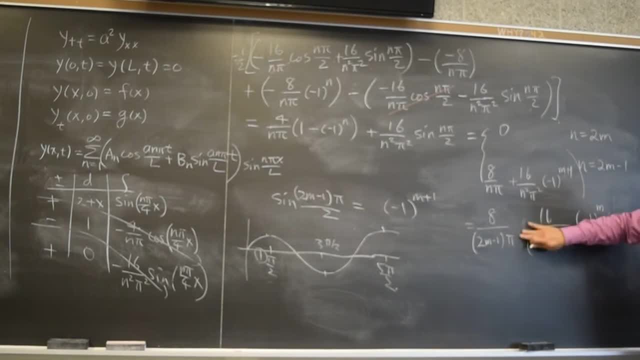 Or, if you want, you can delete this and make this as minus. Okay, Because losing one of the negative 1s you can pull. Okay, So you can rewrite this as negative 1 to the n times, negative 1 to the first power and. 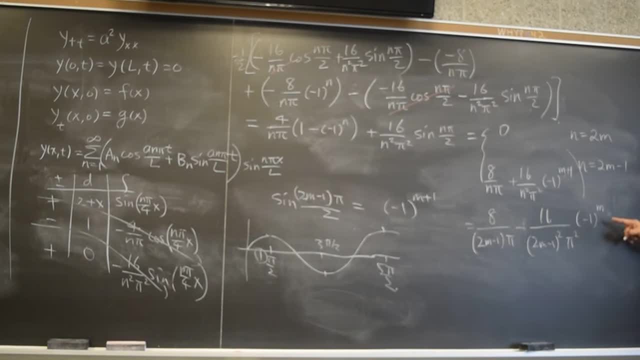 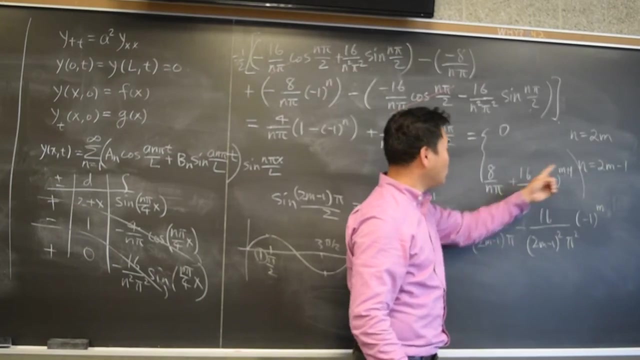 negative 1 can be grown out here. Okay, So that's what we have, And then all that remains is to use this formula. now, That's your an right. an is 0 when n is 2m. an is 2m- an is this thing when n is 2m minus 1.. 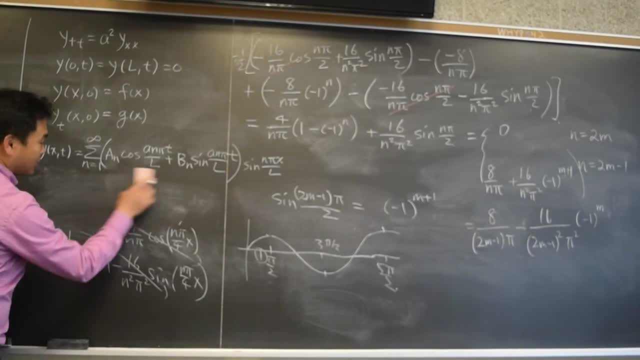 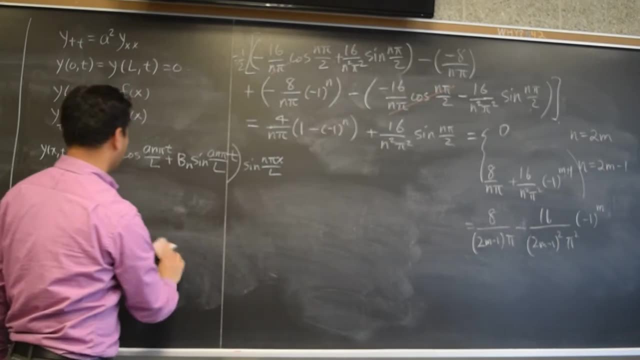 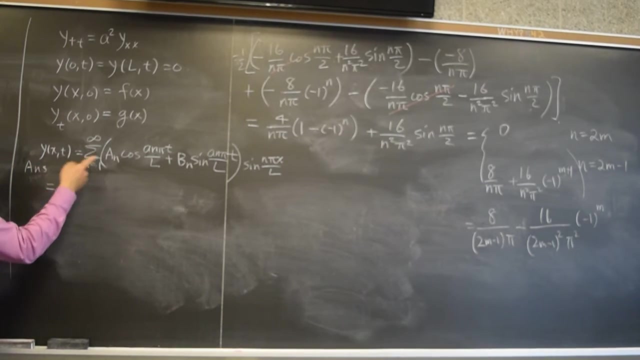 So all you have to do now is to put it here. So the final answer, according to this formula, is sigma. Now we're going to use m, now m from 1 through infinity of a 2m minus, 1 cosine of a 2m minus. 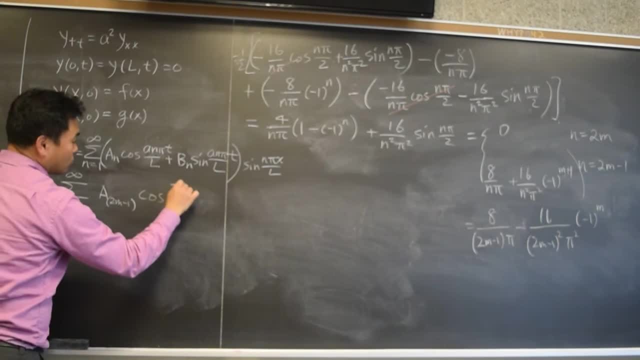 1. Okay, So m minus 1, m minus 1 sine 2a times. Oh, what's the value of a? I raised it but Three. Yeah, See, the original question was given as ytt is 9 times yxx right. 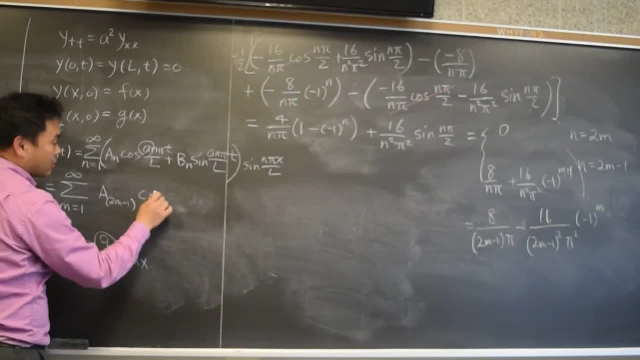 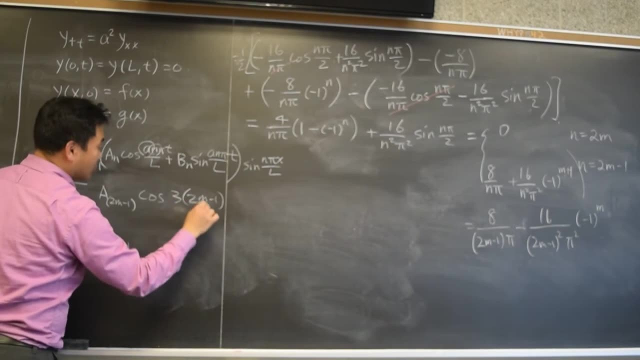 Yes, So a squared is 9,, so a must be 3.. Okay, So it's 3,. instead of n. you're going to put 2m minus 1 pi over. It must be 3.. It must be 3.. 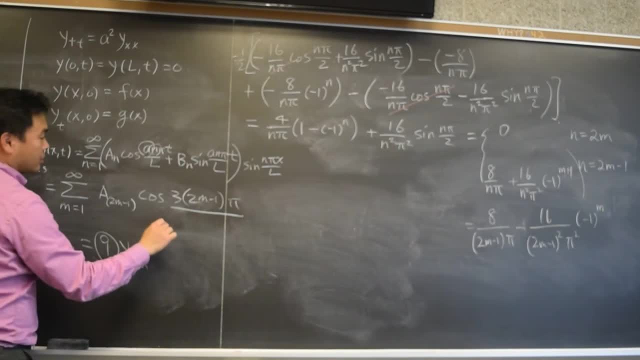 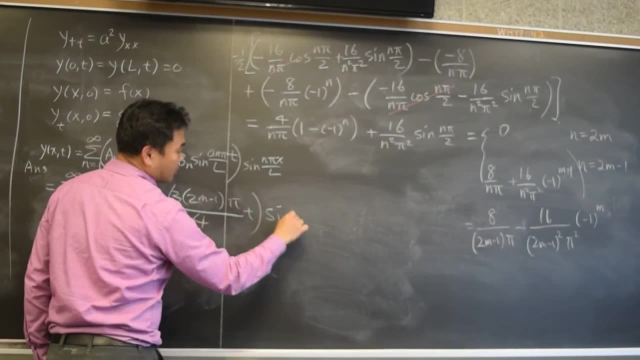 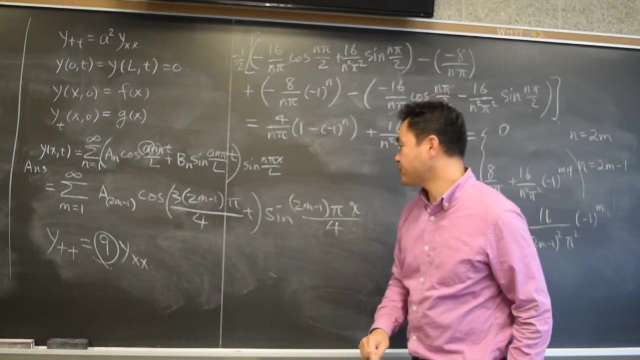 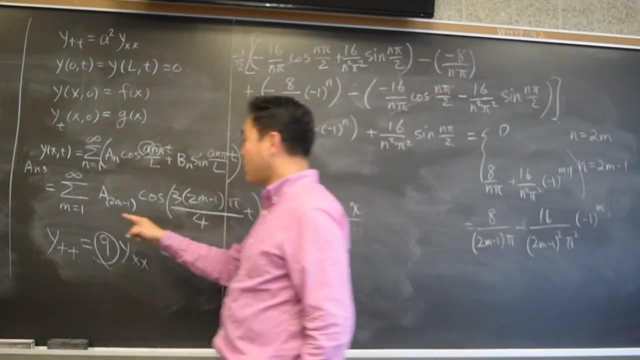 It must be 3.. Okay, over 4t. and then sine 2m minus 1 pi x over 4.. Okay, see how I just wrote down the odd terms. only, Instead of using n, I'm using m, so I only get the odd. 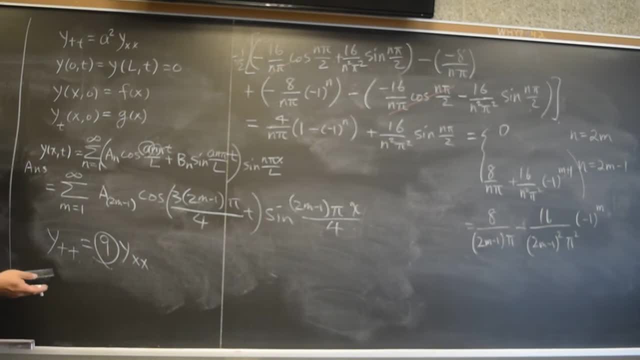 terms. Why is it possible to do that? Because the even ones are zero, so we don't need to put it at all. Okay, and finally, if I quote that and put it in here, and that's the final answer, So the answer is sigma m from 1 through.